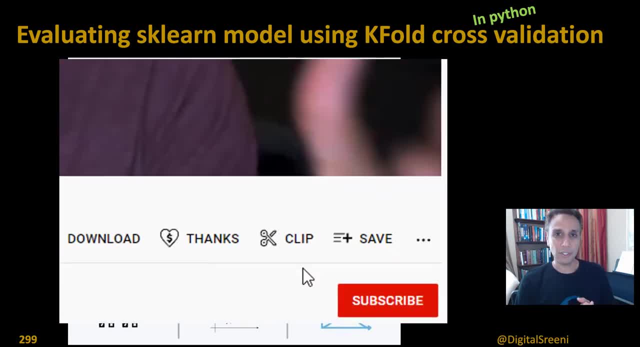 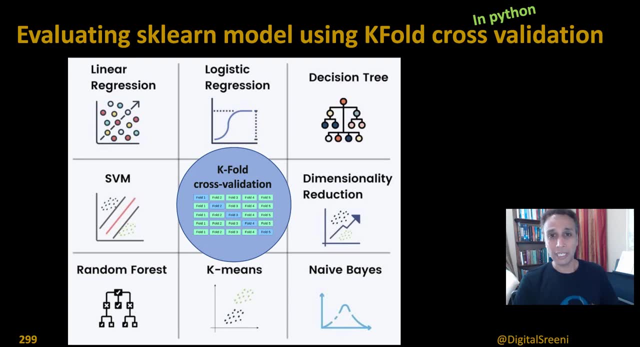 they come out. And if you're feeling extra generous, try to find the thanks button right next to the subscribe button and be generous. Okay, let's jump into today's topic, which is, like I mentioned, evaluating a scikit-learn model. Now, if you are lazy and do not want to watch my 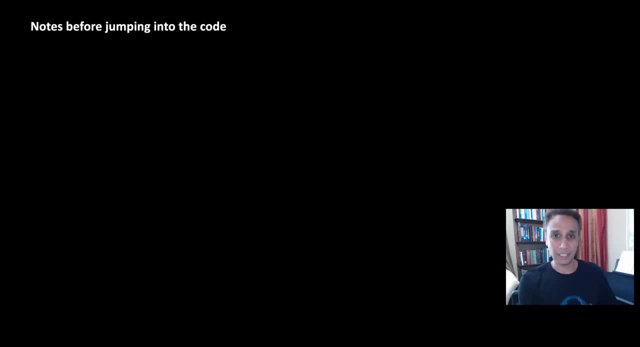 previous video. okay, I still recommend doing that, But here is a quick context, quick background. So what you need to know is that k-fold is a model validation technique. You have a model. you want to know how good is that model for a given problem So you can validate that model for that specific. 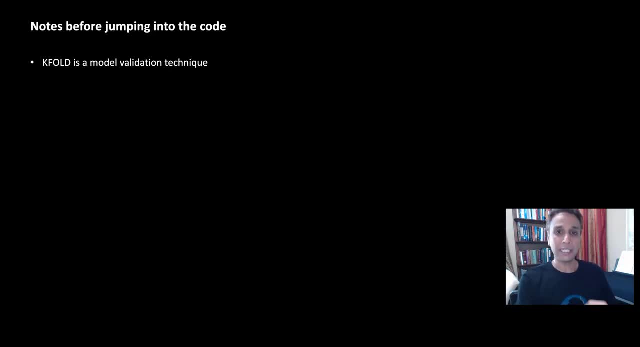 problem using k-fold cross-validation. It is not a technique that will give you a good model. It's not a technique where you can train a model and then get a good model that you can take and use in production for future use. It's just an evaluation. You can use it to kind of find the 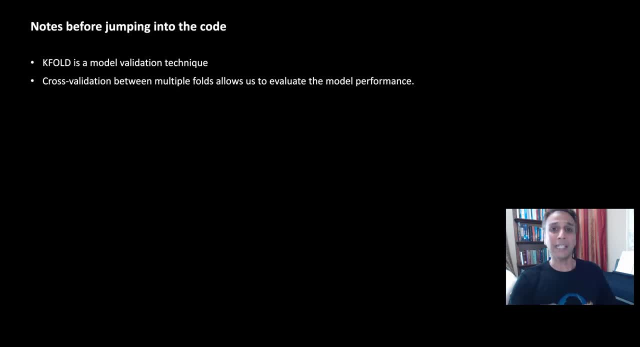 right model and then retrain that later on. But that's the intention of k-fold. cross-validation is not to provide you with a stable model that you can use in future, And cross-validation between multiple folds allows us to evaluate the model performance. So you divide the data into multiple 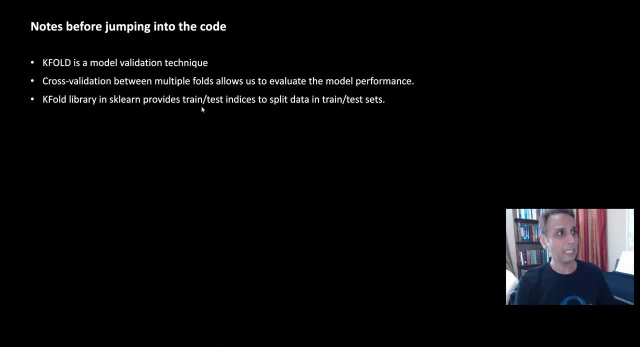 folds. That's what k-fold library does. It provides you the test train indices for your data so you can divide them into different folds. So if you have 500, data points, let me just: if you have 500 data points and your k equals to 10,, then each fold. 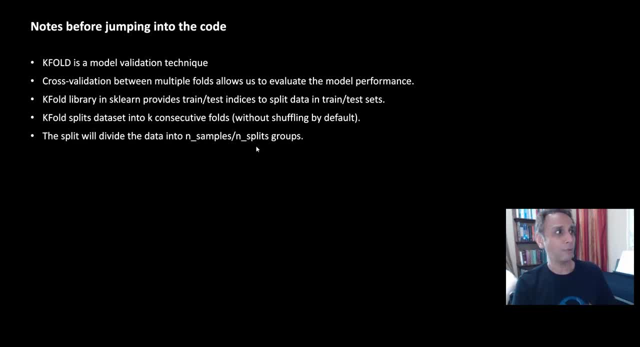 will have 50 data points And of those 50, you would be using one of the folds for testing and the remaining for training purposes. So one group is used for testing and the other one is used for training purposes, And also by default it's consecutive folds. So if you have 500 data points, 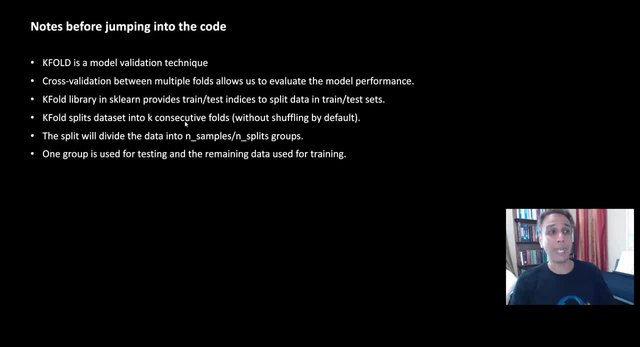 it's like first 50 and then the next 50 and then the next 50. But you can actually tell that you interact with that to shuffle the data, in which case, obviously, the data gets shuffled before the data gets split And all combinations will be used for cross-validation And in this, 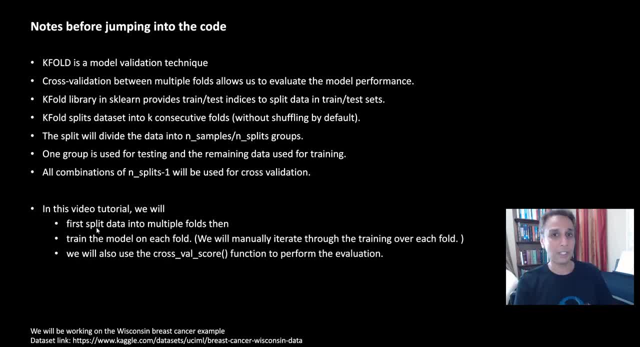 specific video. we will be, of course, working with Python, scikit-learn. we will split the data into multiple folds And we'll do two things. First, we'll iterate through each fold manually, train and validation. Why? Because that's a good way of understanding exactly how. 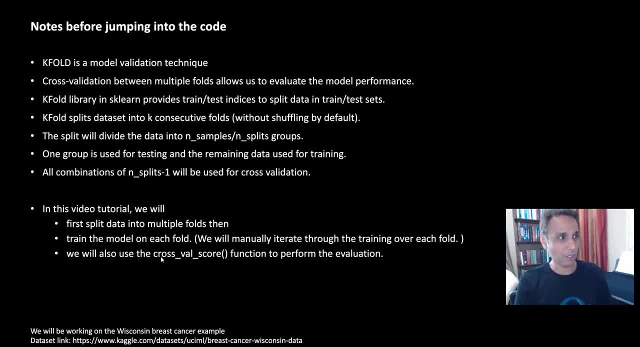 things work in the background, But if you are after one value, which is cross-validation score, which is what just show me how the model is performing one metric, the mean cross-validation score, then there is a shortcut right there. Yeah, there is a method built in method, that's. 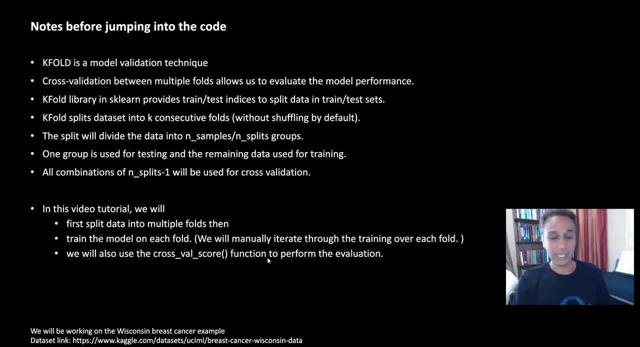 called cross-val score that can be used and we will actually look at that And how do we do this? So I will be using support vector machine and the data set that we are going to use is the Wisconsin breast cancer example. I've used this many times in the past. If you do not know, a quick summary is you have, I believe. 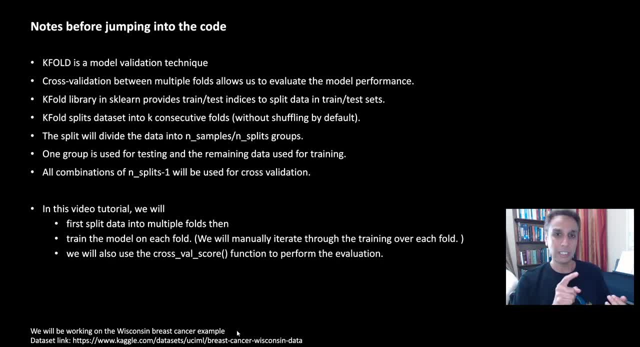 about 30 attributes, which is what is the mean radius of the tumor, I guess, and the texture of this tumor, and so on. So you have 30 such features and then one column that actually shows you what the label is: Is it malignant or benign? So that's the data set right there And it's available. 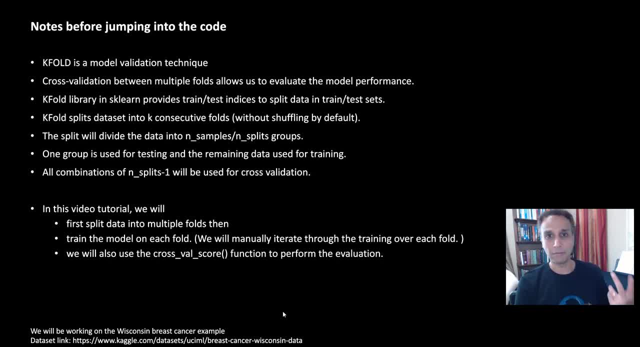 Again, I'll share the link as part of the description So you can. you can download it if you want. It's just a CSV file. Okay, I think we are all set with that information. Let's go ahead and jump into the code. 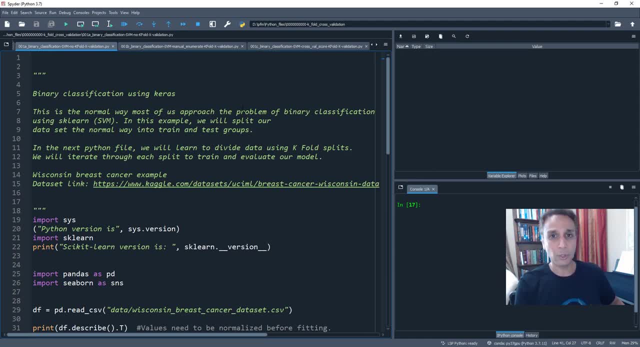 And I do have three files right here. I'll share all of those again. look for the link under the description down below. And the three files: the first one is just a quick introduction to understanding the data set. But, more importantly, okay, if you, if you do. 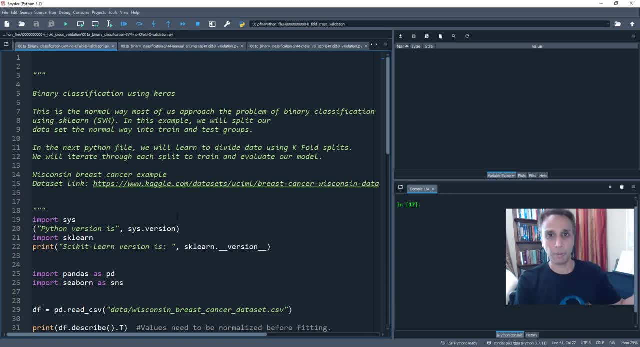 not have K fold cross validation. how would you typically approach this problem? And I did this in the past, but I wanted to quickly repeat this. So you know that, hey, this is the normal way of doing it. But then, with K fold cross validation, this is how we enumerate it through each of the 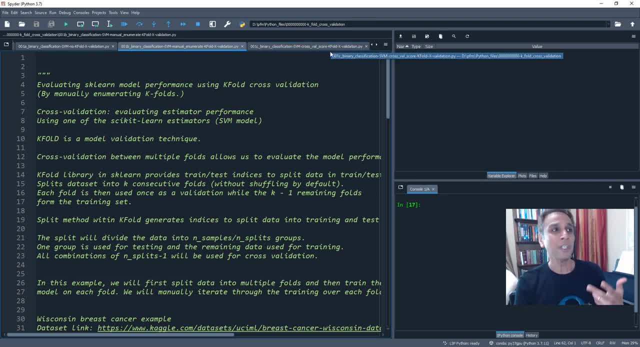 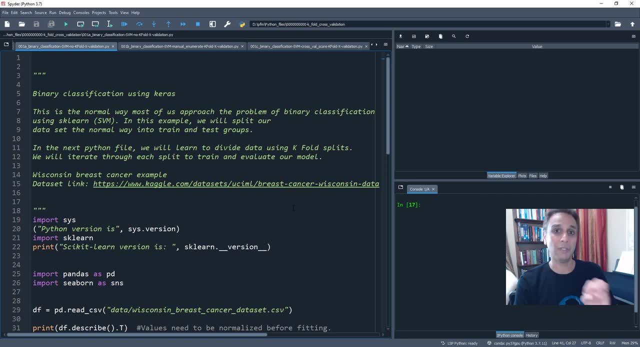 folds using for loop. And finally, hey, shortcut. Yeah, if you are looking for shortcut way, just go all the way to the end of this video, Although you may find some little nuggets of information when you watch this videos- maybe a new way to display data. 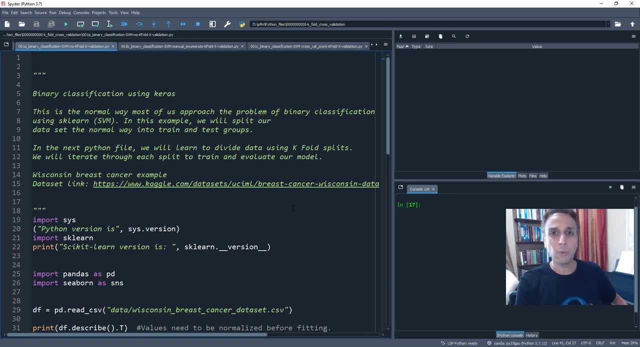 I don't know, but try to watch the entire videos And also try to watch the advertisements, because it provides. it provides money that I want to donate to charities. Okay, guys, with that, let's go ahead and jump in. And here is the information. So let's go ahead and import this. 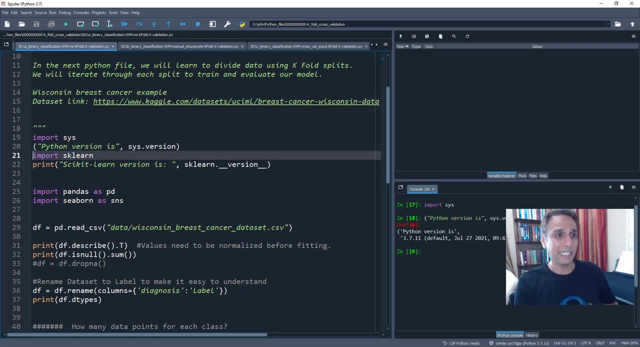 so I can print out exactly what my Python version is. It is 3.7 dot 11.. And I'm using scikit learn. we are going to use scikit learn and the version here is 3.7 dot 11.. Let's go ahead and import pandas, because we need to capture this table that I 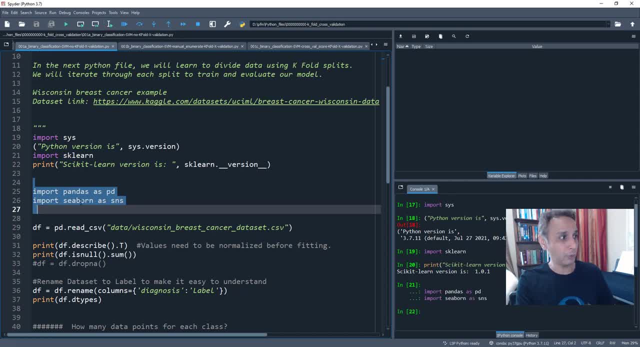 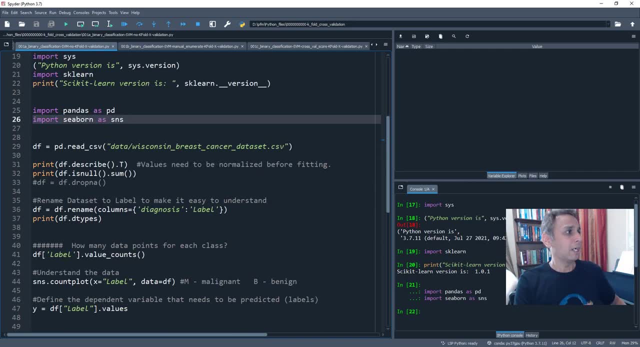 showed you the CSV file as a pandas data frame, And I am going to also import seaborne, our pipe plot. it's up to you, So we can quickly understand how the data looks like. Okay, now is the time to read the CSV file and store it as part of a data frame. So let's go ahead and do that, And when I 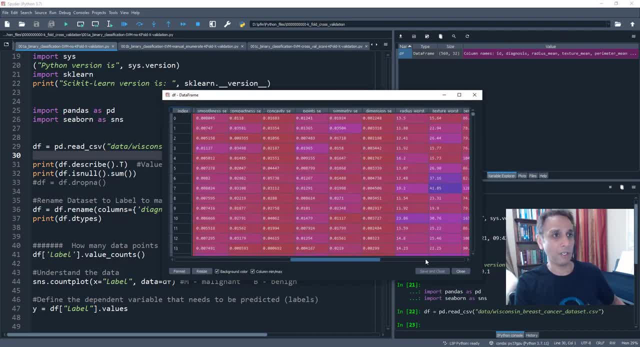 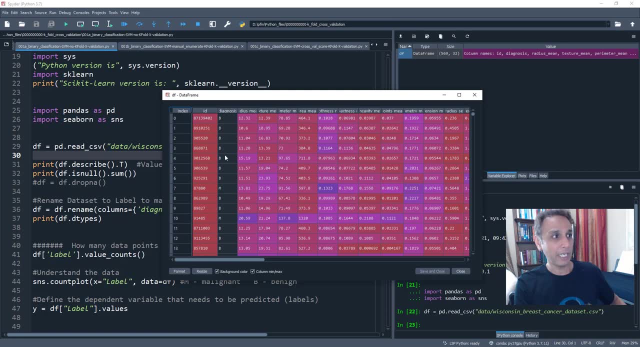 open the data frame, you should see that I have a whole bunch of columns right there. I believe about 30.. One because one of those is diagnosis right here, benign or malignant. So this is our label. I don't like the title diagnosis for multiple reasons, Because one reason is I it's. 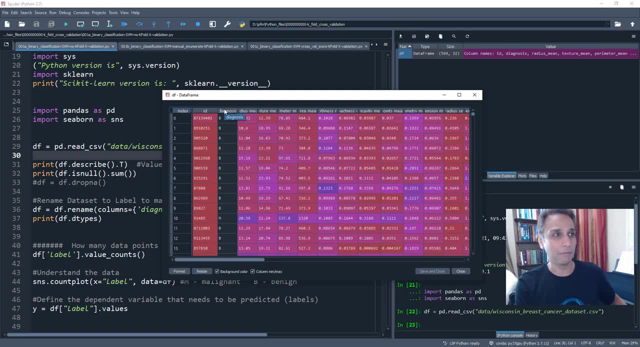 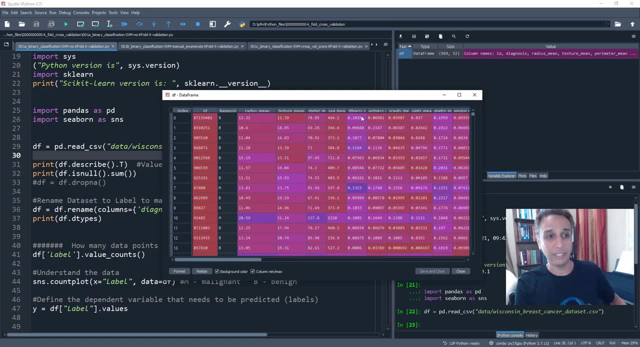 hard for me to say it, So I'm going to replace that with a label called label, Easy right. And what other attributes do we have? radius, texture and so on. Yeah, so there's a whole bunch of attributes. Again, look at the documentation for this data set to understand what it really means. 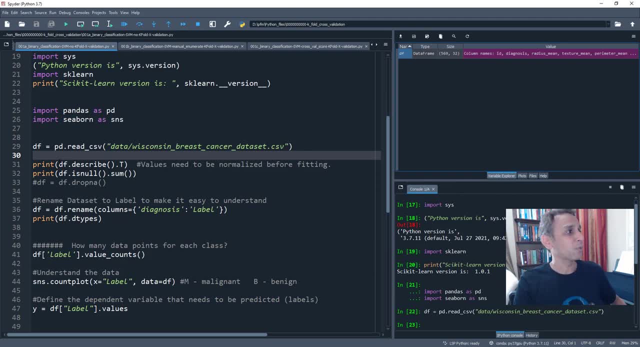 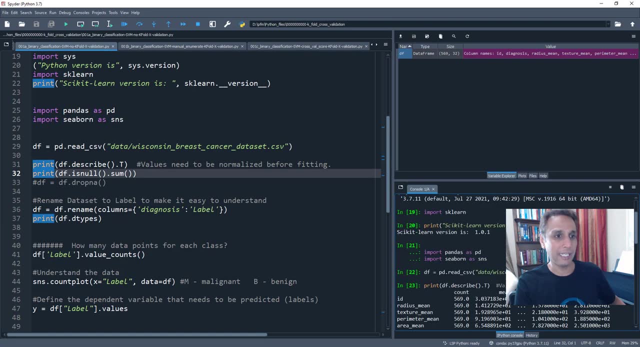 But let's understand the numbers first. So why? let's describe the data set we should have, Yeah, 31 rows, eight columns right there, And we have 569 data sets. And these are all the attributes, not data. 569 data points, And these are all the attributes: radius, texture, perimeter, area, some. 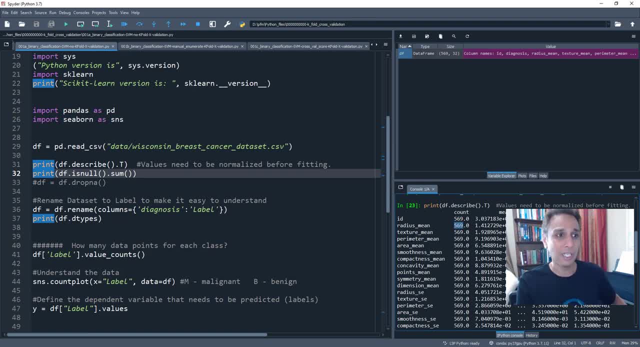 of these are related, right. Obviously, these are not independent. parameters like perimeter and area are probably, The radius are probably related, unless they're measured in a different way. But I can't understand why that would be. But anyway, so there is concavity and all of these other parameters. So 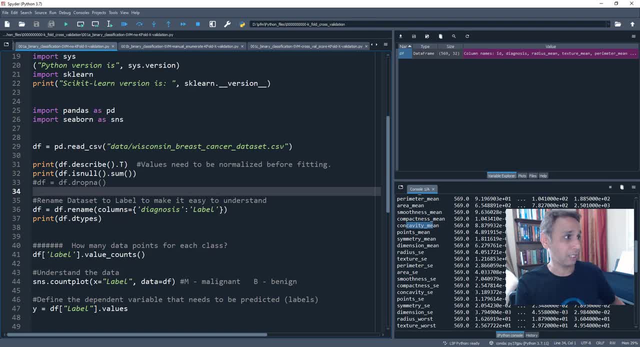 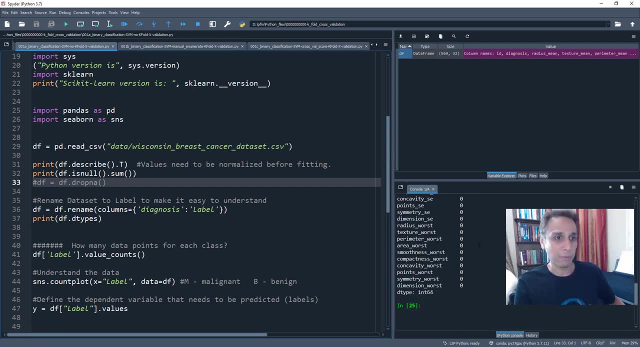 how can we fit that to a support vector machines model? But first thing first. are there any null data points, right? So we need to take care of those. We do not have any, so not much to do. Otherwise, I usually drop any null rows or fill it with some values. But 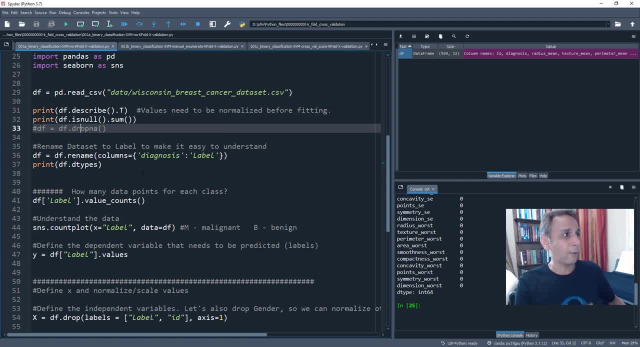 they're the same And we'll just assign kind of a one or two and then that will actually be considered null. that's what we're already doing, But yeah, it's up to you. Okay, now I already mentioned I would love to rename diagnosis to label. Let's do that. And now let's finally look. 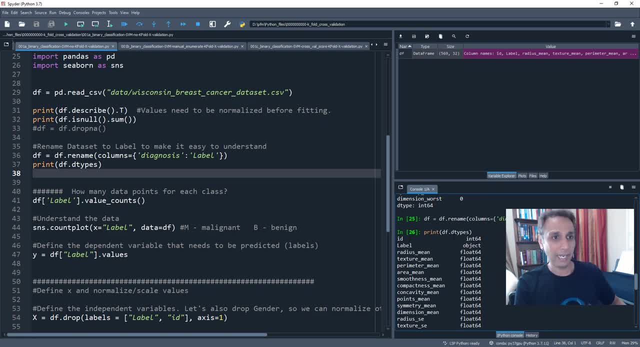 at the data types, And everything is a floating point value, except for a label, which is an object. Of course, our label is M or B, So it's a text, it's not a floating point, it's not a number and our ID is an integer. Okay, and let's understand the data point: How many malignant versus how many billions you can get? 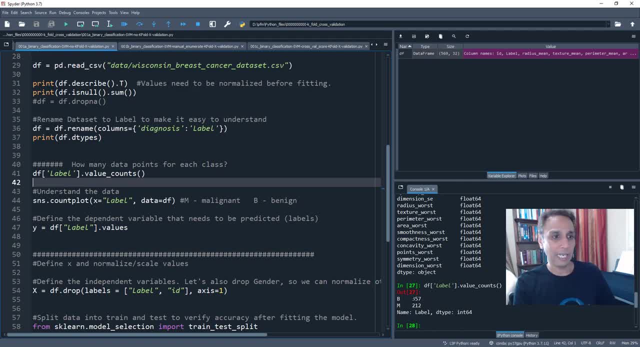 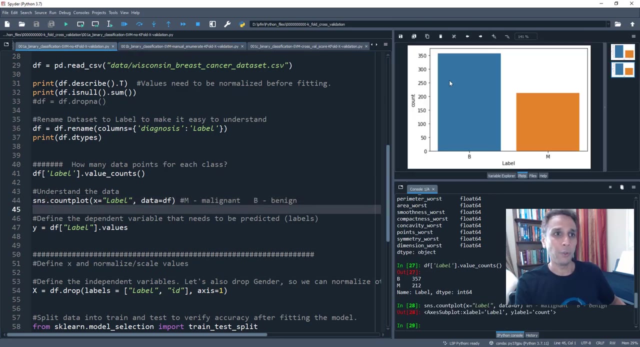 do we have, so let's go ahead and print that out. we have 357 benign, 212 malignant, so it's not really that balanced. if you want to balance it, you can go ahead and do that and the same information. if you want to plot it visually, you can understand how it looks like. there you go. so more B compared to 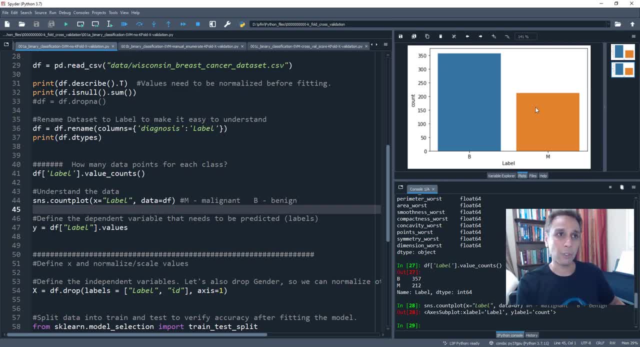 M, and you can watch my one of my previous videos where I talked about data imbalance and how to balance it. what type of different techniques do we have? again, that's a different discussion, so I don't want to get into that, but if you want to do that, this is the time to do all of that. okay now. 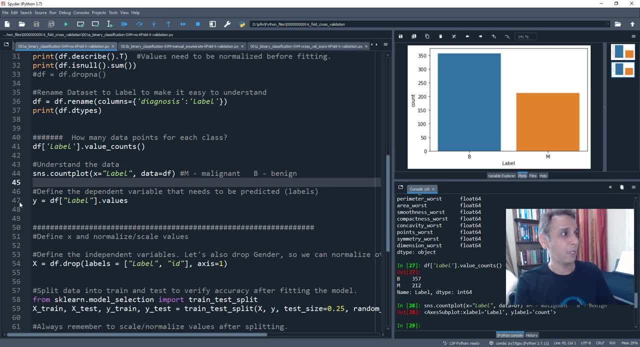 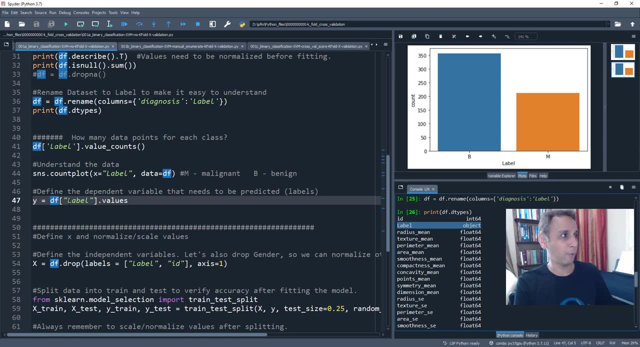 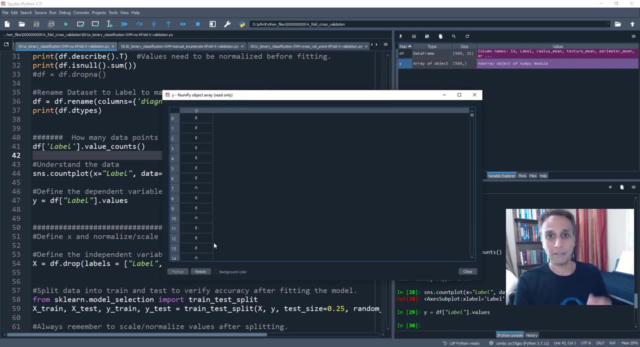 let's define our X and Y values for our machine learning. so why? is very simple, it's nothing but the label right there. so that column, so that is my Y. so let's go ahead and extract that and if you open this or Y, you can see it's that. 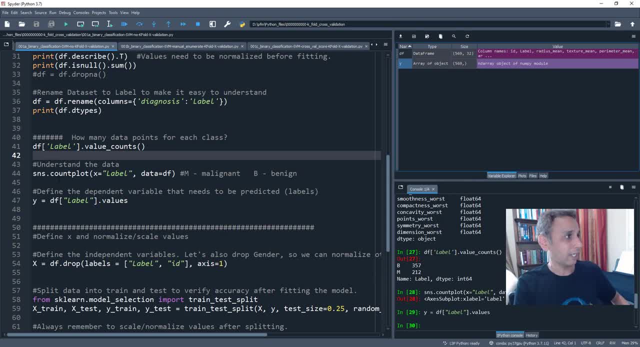 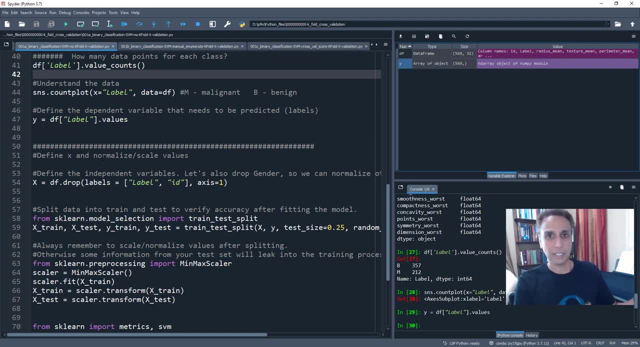 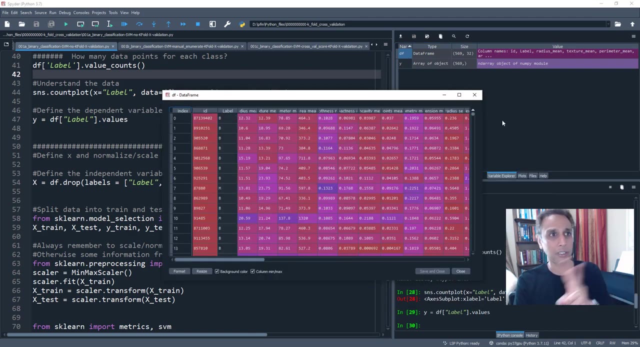 single column that we extracted. so now, this is an area object. now let's go ahead and define our X. and our X is all the columns, except for the two that that are not attributes, ID and label right. except for these two, all the other columns are our X values. if you want, you can pick and choose which ones. 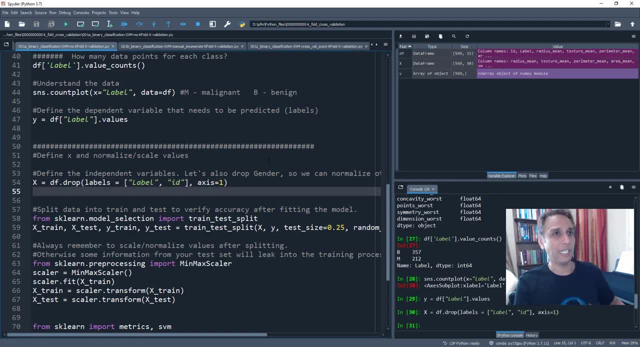 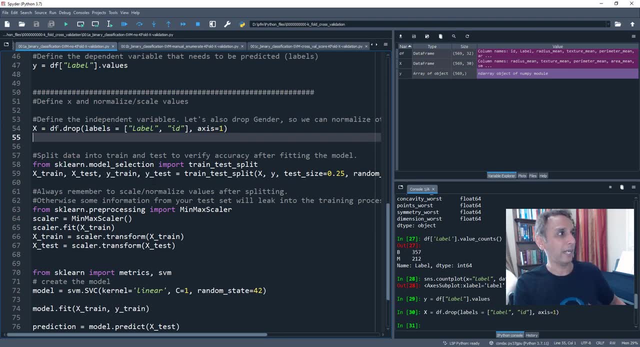 you want to use, so let's use the remaining 29 right there. so there you go, okay. so now that we have our X and Y ready, typically, what the we do, we use our scikit-learn model, selection, train, test, split and we split, split or data into. in this case, I am using. let's do this. in this case I am. 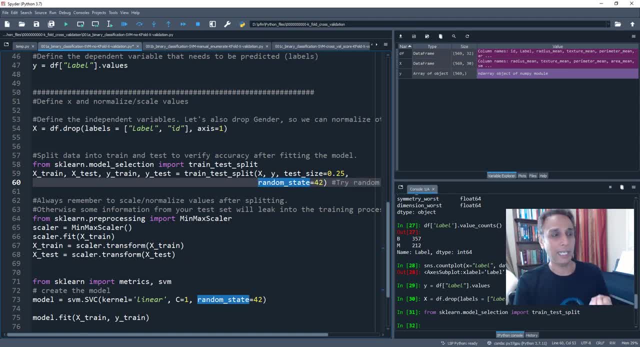 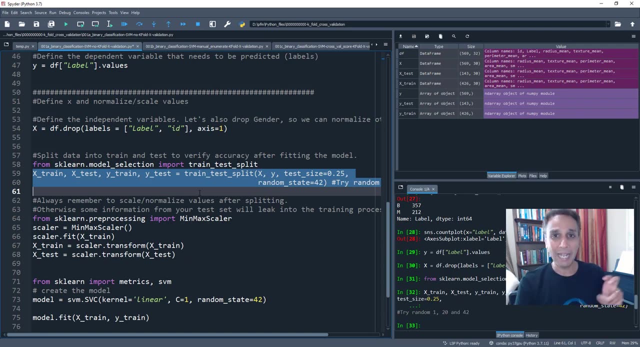 using 25%, holding 25% of my data as for testing and the remaining 75 for training. so this is how we typically do. let's go ahead and do that, in fact. let me also mention one thing. I used to do this bad habit. I used to have this bad 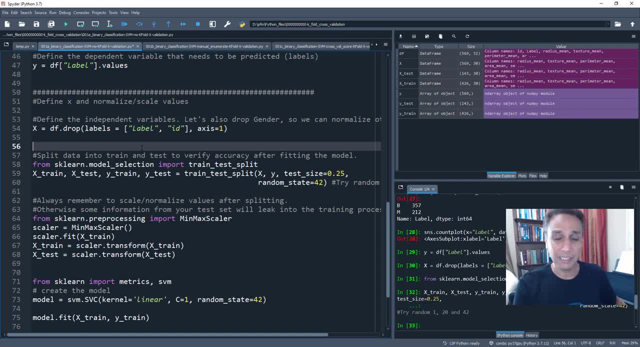 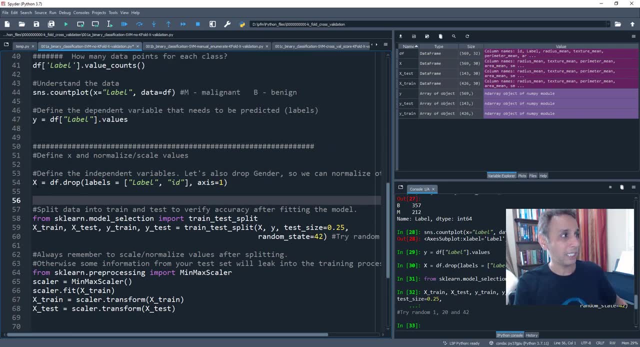 habit of normalizing or scaling the data. talk about little nuggets of information when you watch the video. if, typically, i used to at least normalize my values right there, or scale the values if you want to call it, like, for example, min max scalar or standard scalar, etc. right there. 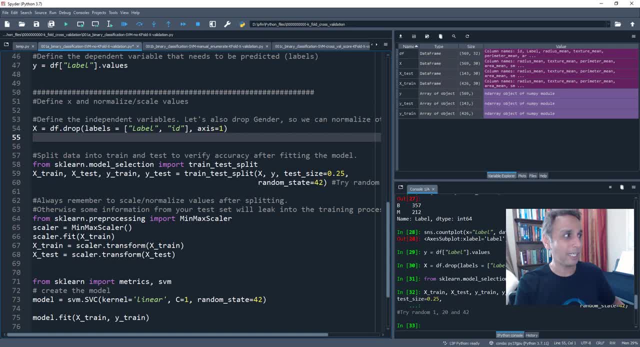 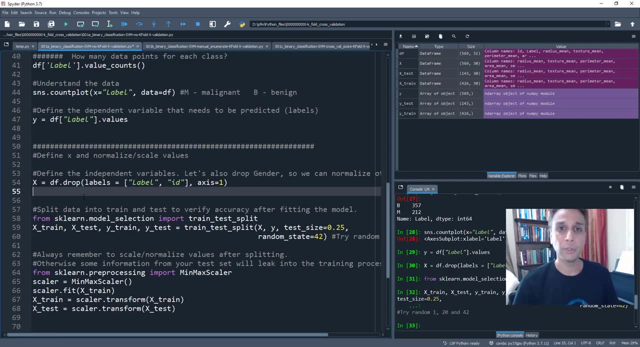 and then split the data. never, ever do that, never do that, because always, first thing, remember to scale and normalize after splitting. because what happens when you do your scaling or normalizing? well, you are, for example, if your x data has data that goes from 0 to 100, and when you normalize, 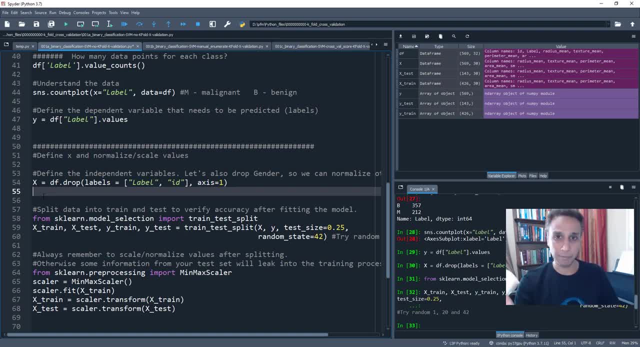 the entire data. it's like normalized to 100. right, so that's the maximum if you're doing min max scalar. but when you split it, what if your x train has only the the highest value to be around 75, but then x test actually has the values up to 100? then your data mean and the standard deviation is different. 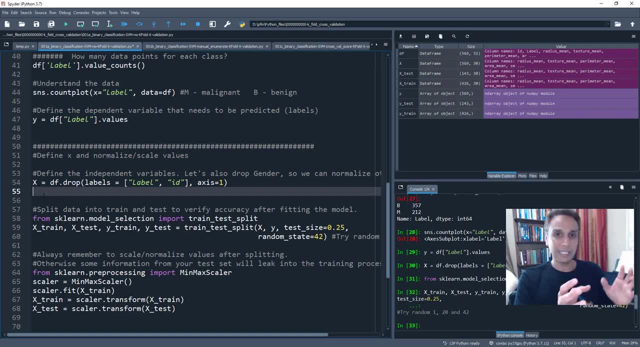 between these two. so when you normalize and provide that information during the training process, when you normalize ahead of time, then the training already knows what the spread looks like in your test data. so some information from test is leaked into your training, which is not ideal, right? so that's why you need to. that's. 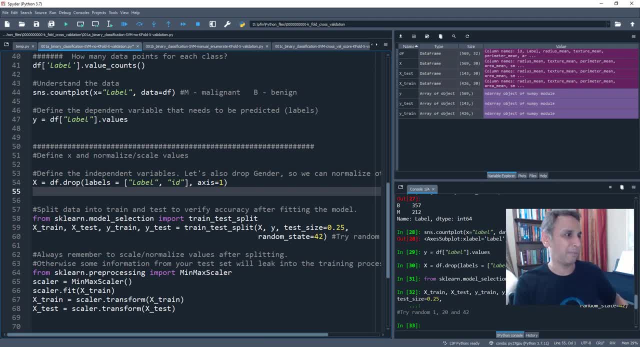 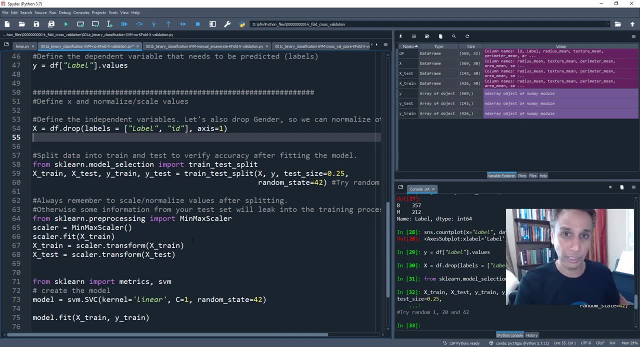 … that's. I think there's a term called yeah, it's basically. the information is leaking into the training process and I added the notes right there, so that's exactly why you need to be scaling them after the split. so we did split here, so 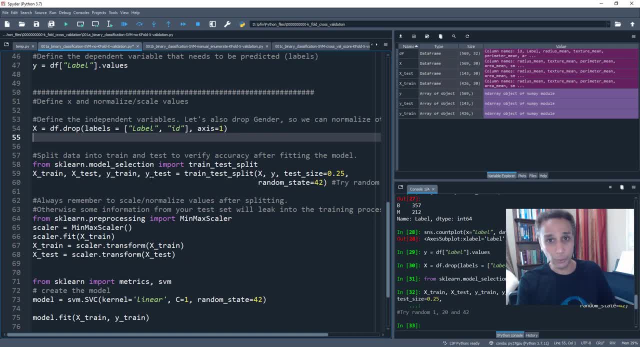 we have our x-ray and x-test, y-train and y-test, and why you're not doing anything. I mean you can convert them into integer encoded, because right now we have M and B. you can convert them into integer encoded or one-hot encoded, if you are. 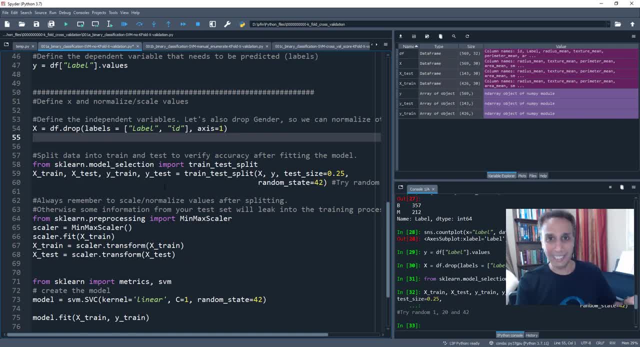 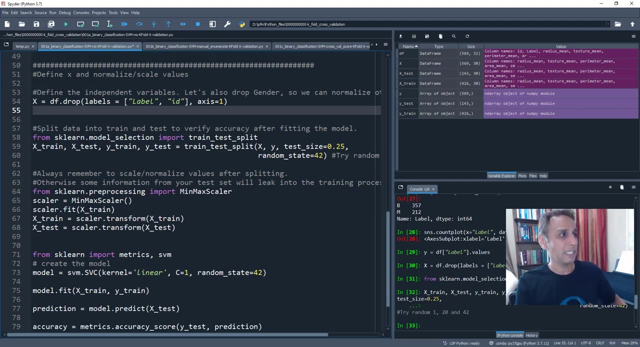 doing neural networks, but you know, in this case we do not need that support vector machines and random forest. they can handle these type of text, textural labels, so let's leave it as is. but our X values. we are going to scale them and I am choosing to use min max scalar in this case, again available as part of 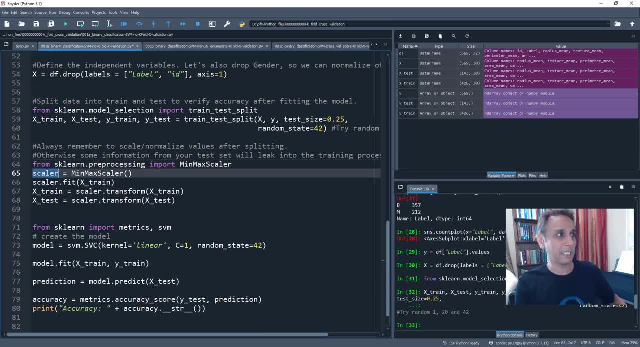 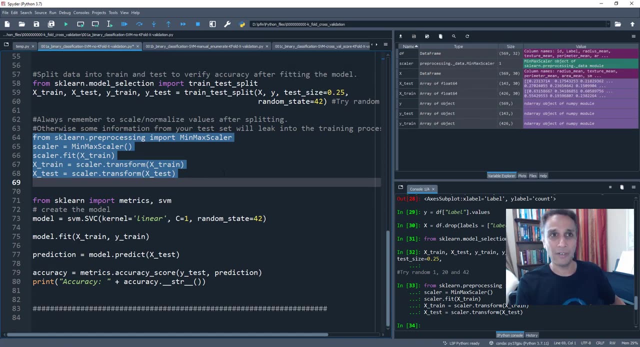 scikit-learn the way you do that is, you define your scalar object and you fit it on to the data and then you kind of scale and transform your, your test data or whatever the future data is. so let's go ahead and run these lines and now our data is all ready. okay. 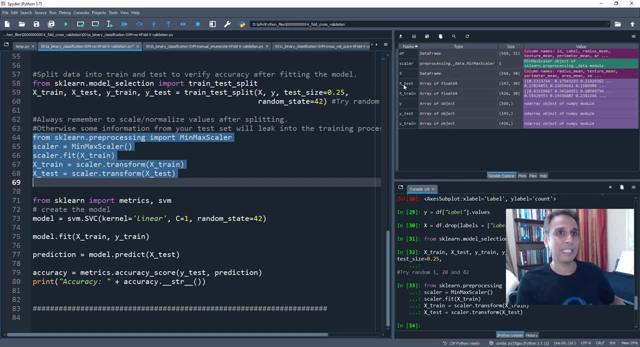 so our X right there. X test. as you can see, the values are now 0.2 instead of. we should have looked at the numbers before. I said instead of, but I have no clue what it was anyway. now let's go down to this: is this is how we used to fit right. 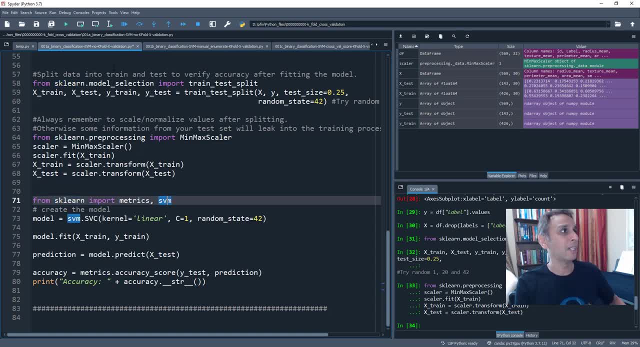 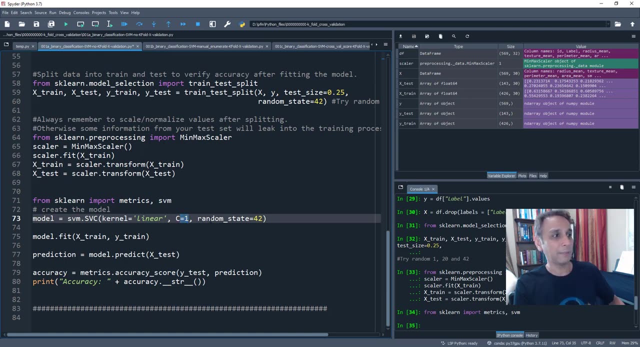 I mean you have your support vector machine SVM and SVM, goddess. BC, our kernel. we are going to use a linear kernel. you can use a cross-validation here. I mean I'm going to use cross validity, not cross-validation. sorry, our C value right there equals to 1. there is, there is no. 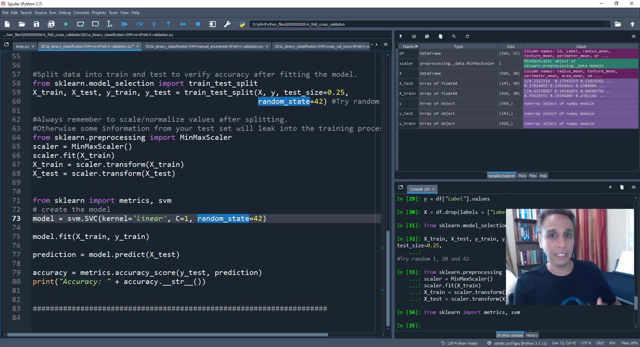 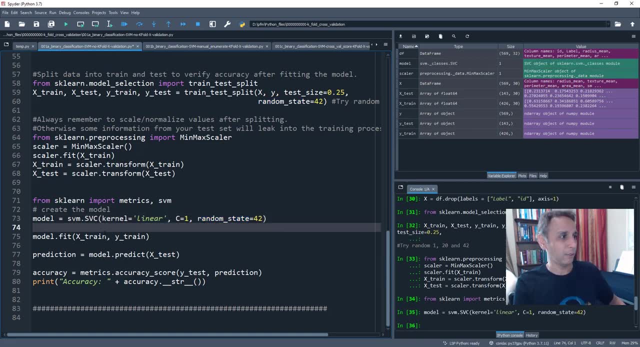 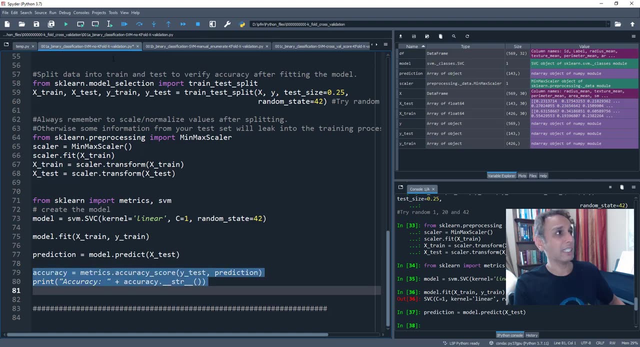 cross validation within this SVC. we will do that in a few minutes and you set your random state and let's go ahead and run this and you fit your model and you predict your model model and you print out your accuracy, right. so this is how we do it and I got. 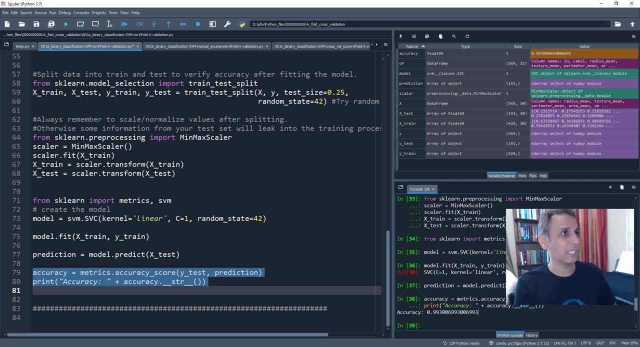 ninety, nine, point three: great, but what if I shuffle the data? what if this gets split in a different way? for example, if I split this, I don't know. ten, yeah, so let's go ahead and run all of these, and what? how does the accuracy look like now? 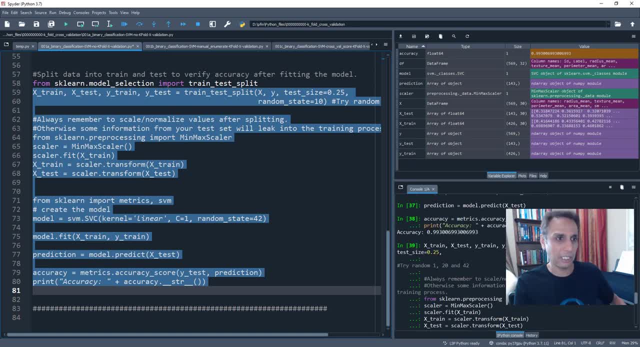 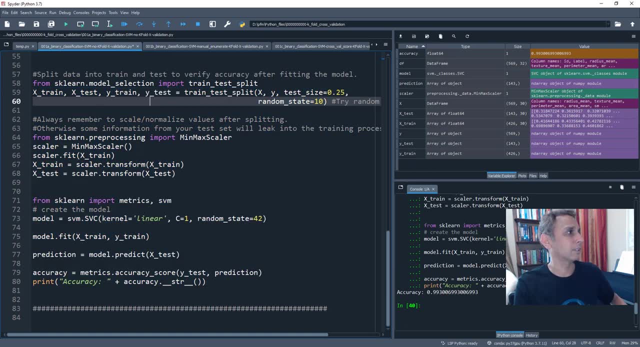 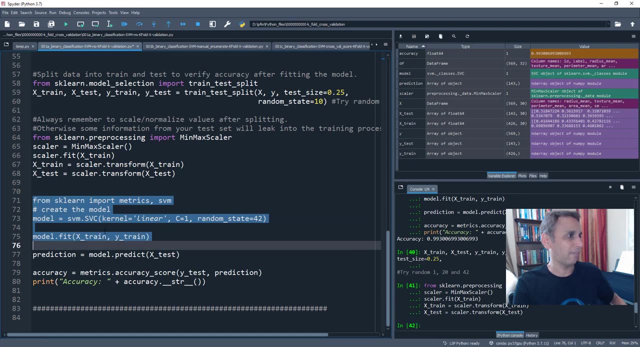 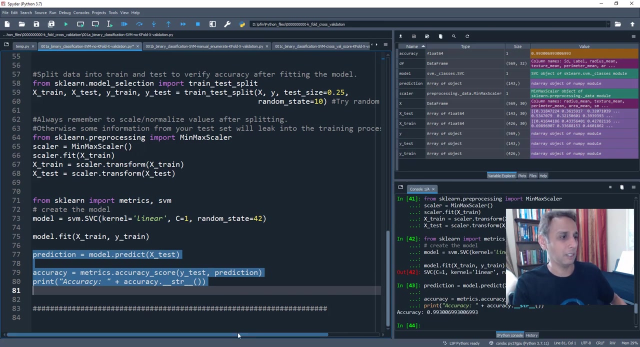 I got 99, point three. what did we get 99? is it doing anything? let's do this in a nice methodical way: there you go, there you go and model dot fit. I was expecting different values, but ninety nine point three, that's a surprise. 120, 42 probably. 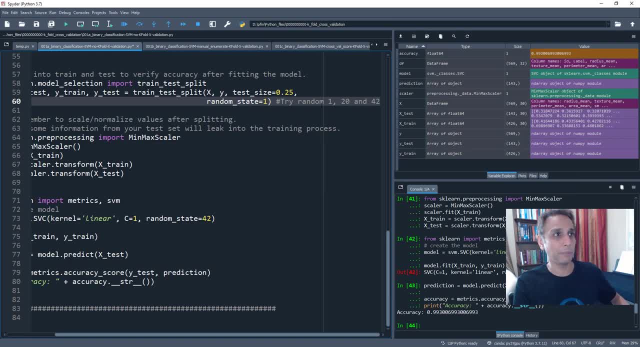 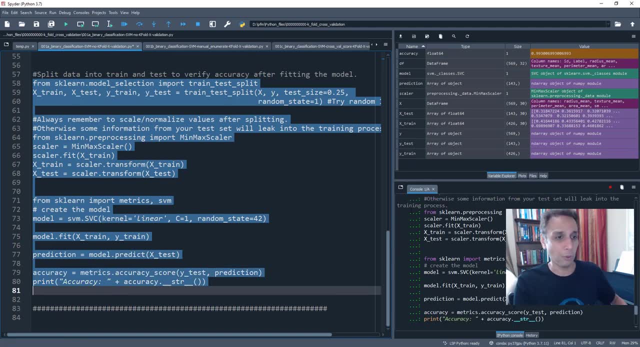 10, split it in a way that's very similar to the previous one. I was testing these, so let's go back to these and check this one more time. hopefully we'll see a different value. otherwise, I have no clue what what's going on. okay, that was a. 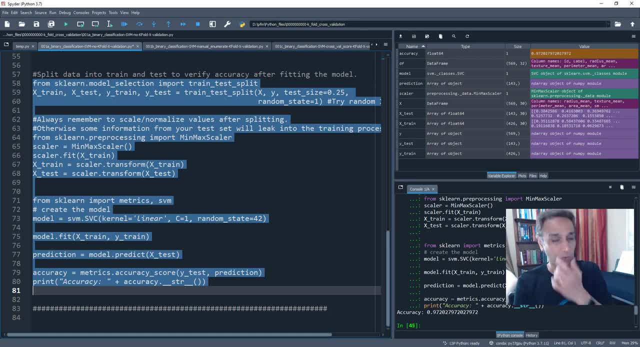 weird coincidence, the way my random state equals to 42 and random state equals to 10 was splitting the data in a very similar way, so I got the similar accuracy. now I split it in a different way. I got 97.2 instead of 99 point. 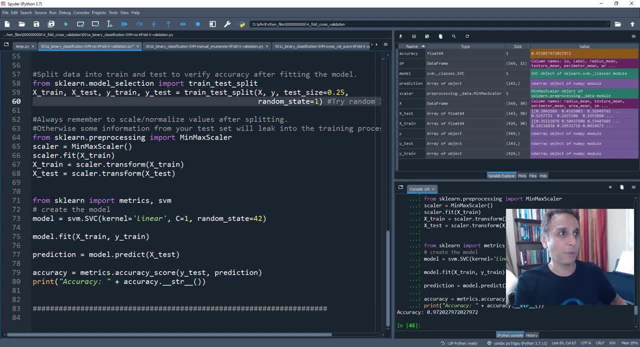 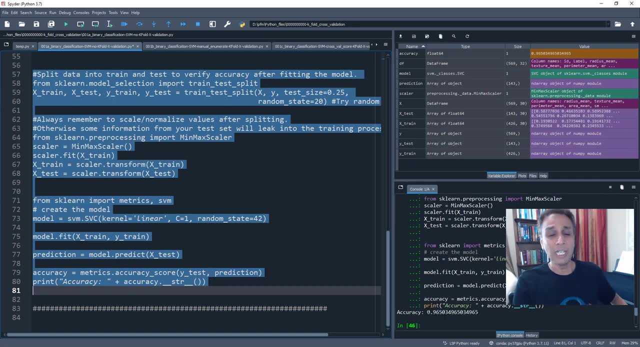 something I also tried by 20 right. so let's try this one more time before jumping on moving further. so there you go, and what did we get? 96.5. so, as you can see, as you change how the data gets split, your accuracy is changing and K 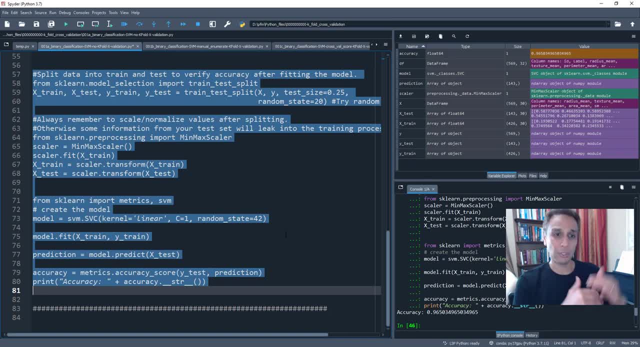 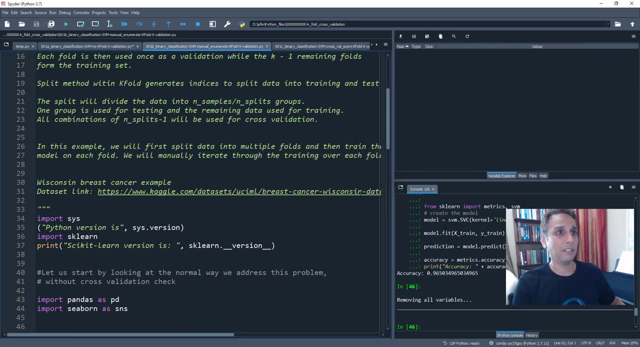 fold is just a methodical way for us to actually split the data in a structured way, not a random way. this is the random way, right that we tried, and then evaluating the model. that's exactly what we are going to do here. so let me clear everything right there and start from scratch. I'm not 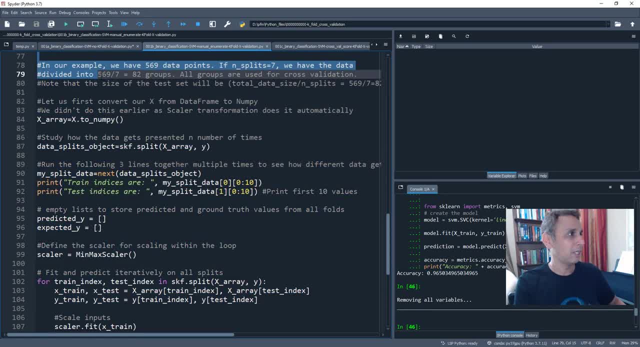 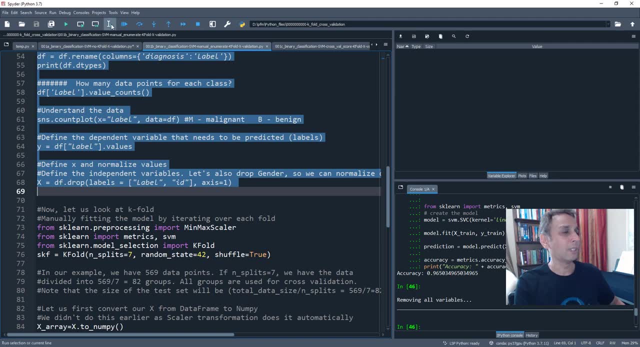 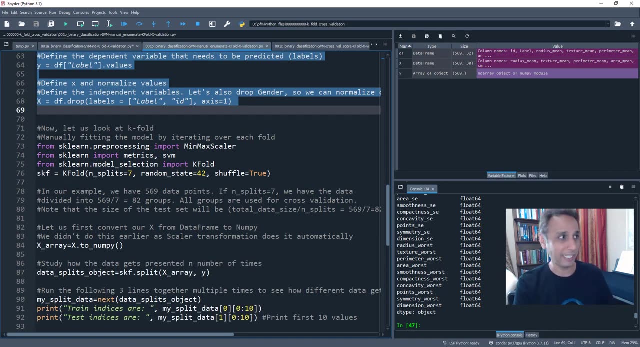 going to explain everything all the way down to down to where we have our X right there. so so far, what we have is just define our X and Y, that's it. and from this point on, how do we do our K fold validation? first thing, first again we. 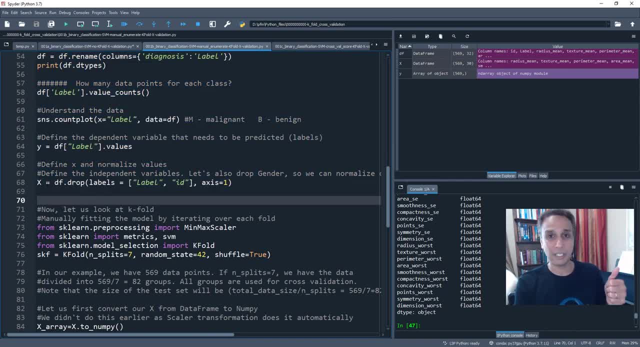 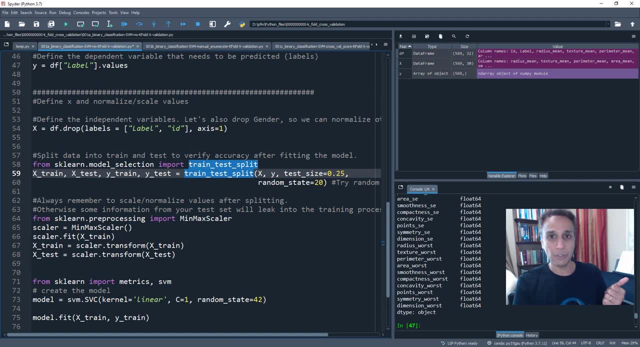 need to perform here. I did not do any min max scalar because previously we did the split. we did the split right there and we are scaling the values. but right now we are we are not doing the split, we are letting the K fold do the split, so we have to do the scaling after the fact. 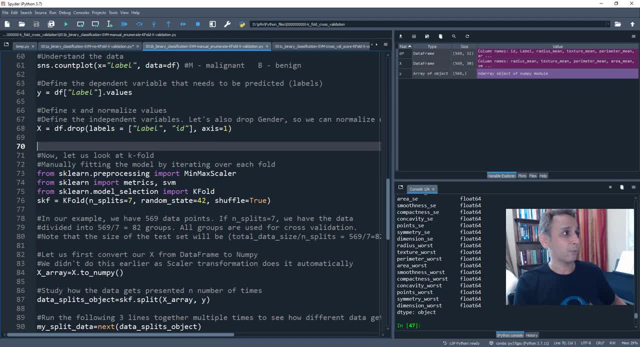 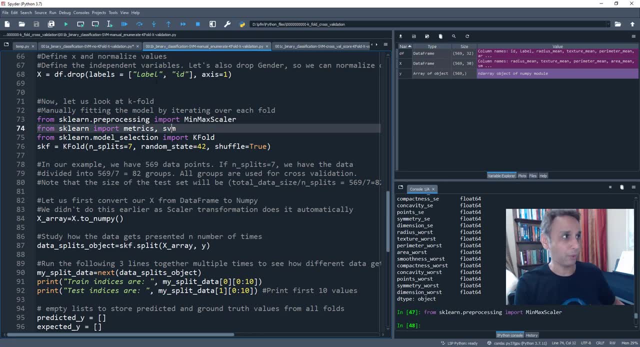 after the split happens. yeah, so that's just a quick note. that's why I only have X and Y. that's it now. I want to import them in max scalar library. I want to import my support vector machines. in addition to that, I want to include import my K fold. it's available as part of scikit-learn model selection. 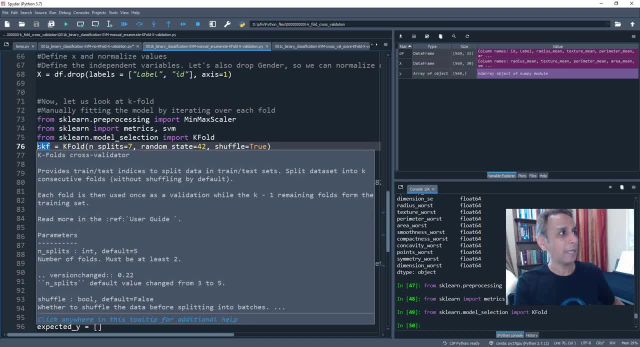 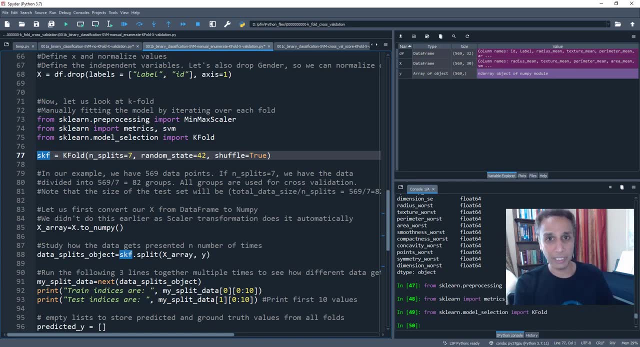 so there's go. there you go, and I am creating my K fold object right there. so SKF is K fold. how many splits do I do we want to split this data into? so let's select a number of splits equal to seven. it's customary to use ten or five. 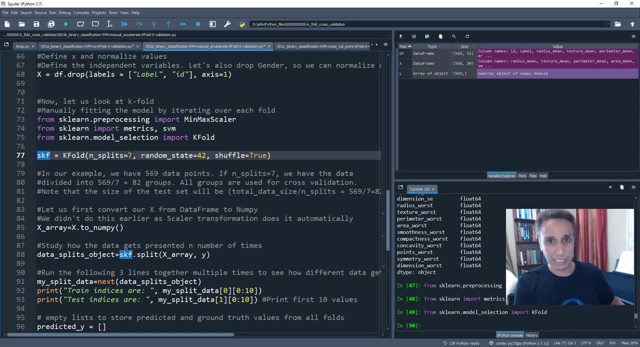 sometimes in between five and ten. so let's just do seven splits in this case and random state. whatever the random state you want to keep, keep 42 is the ultimate answer to the ultimate question of life. so that's why I have 42 right there and I'm going to leave. shuffle equals to true. I want to. 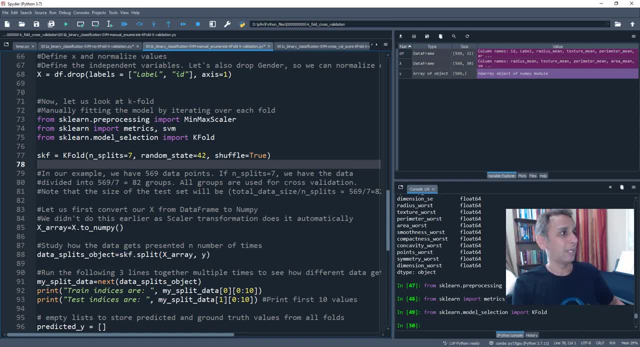 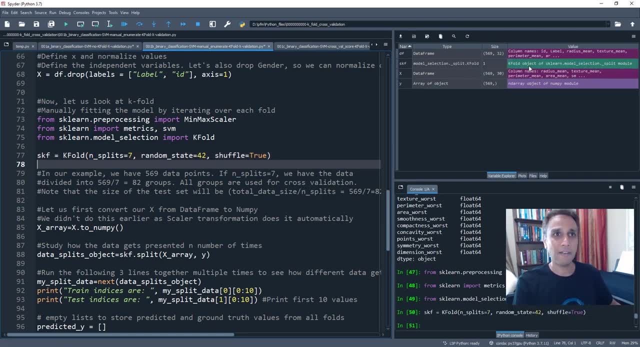 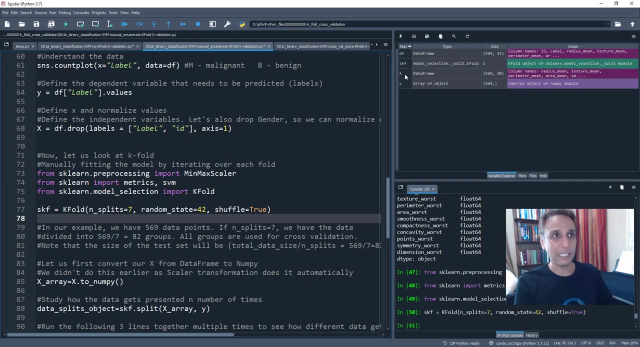 shuffle the data and then do the splits. okay, so let us go ahead and run this line and now you can see: the SKF is the object, K fold object. now we need to use that object. how do we do that? so, first thing first, our X is a data frame, right? 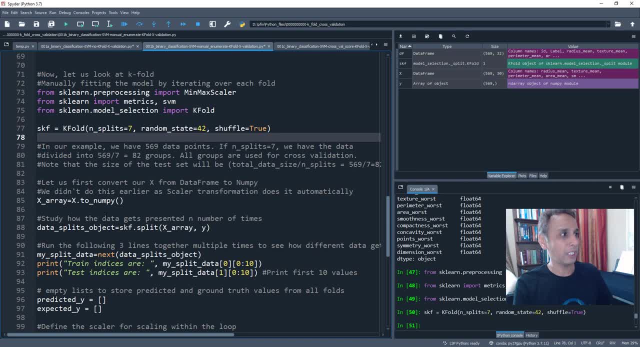 there, so that doesn't work. in our case, we need to. we need to convert that into a numpy, and you can see that we need to convert that into a numpy, so we need to. ch守 đ y xaray, shouldn't, would you? you know how to do that? 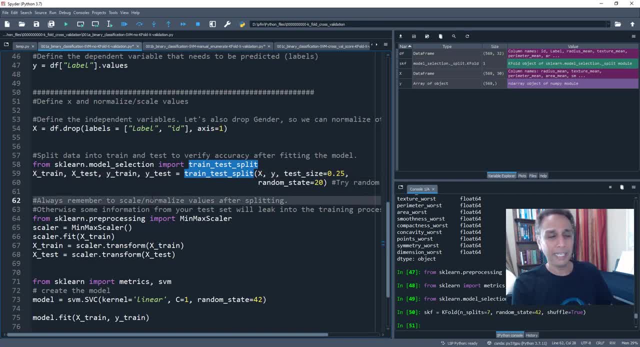 xaray x to numpy. so let's go ahead and do that. and why didn't I convert that in the previous case right here, and these are basics of Python. I didn't do that because when you apply Minmax scalar, it automatically converts that into a numpy. 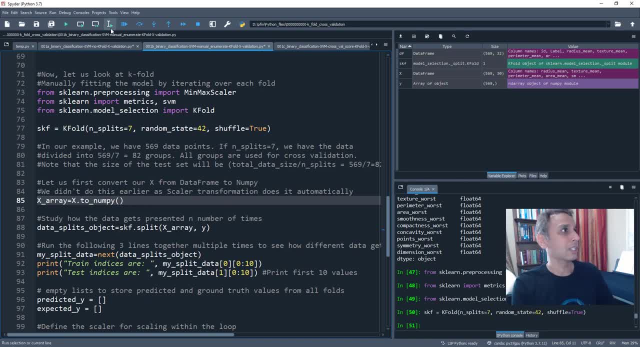 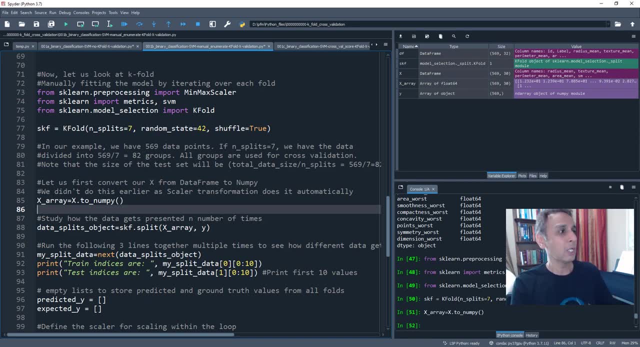 array. that's why I didn't do that. now I have to do it deliberately. that's why I'm trying to change that to numpy. and now, if you look up here now, we have an array of 3569 by 30. okay, so now let's go ahead and create a split object. so our 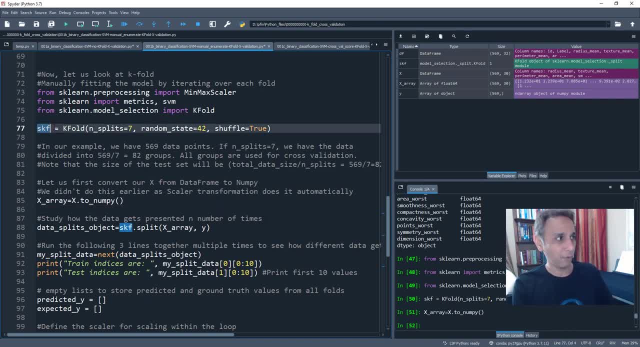 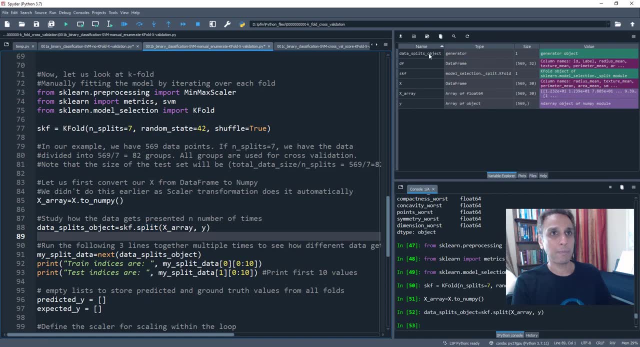 SKF operations run here and I 부동 tomb ra do. I'm going to just do the same thing here. skf object right there, k fold dot split with this input data. so when i do this you should see my splits object being generated and again, i encourage you to understand exactly what that split object. 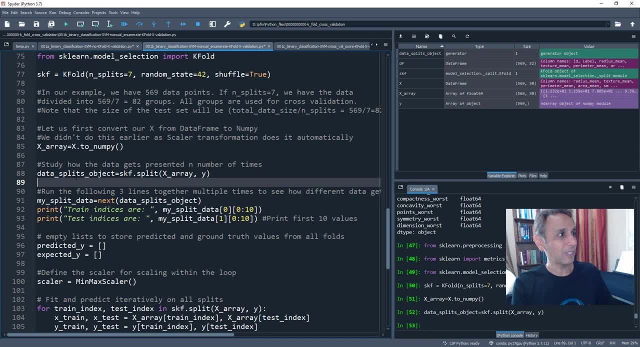 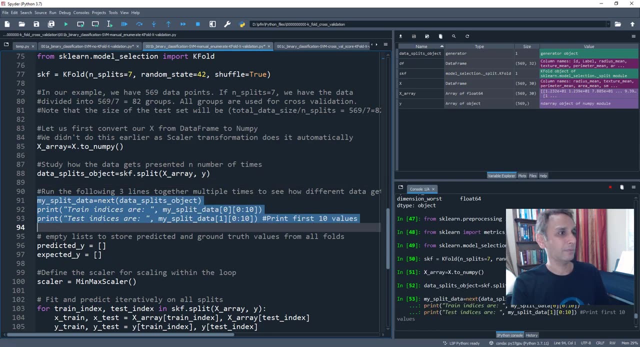 does. that's exactly what these two, three lines are. so this is a split object that walks you through individual folds. so if i just do my next, yeah, walk through these individual folds and look at the split object and go ahead and print out. let's go ahead and do that, right there. i'm printing only. 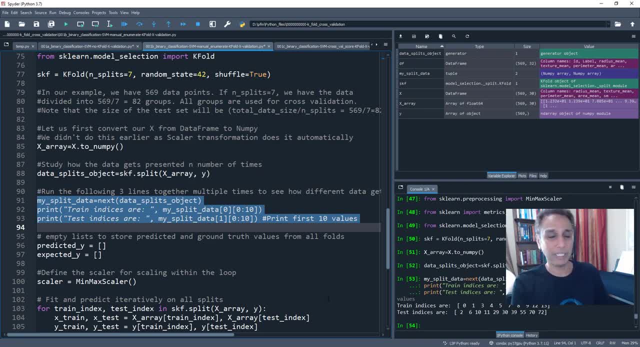 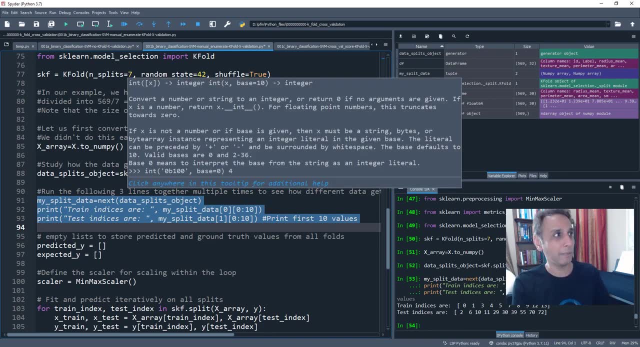 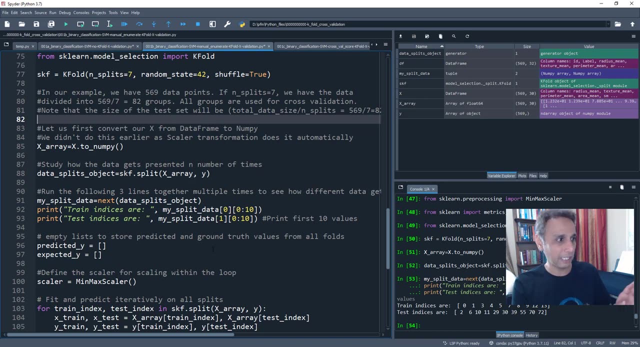 the first 10, not all the 82. uh, right there. oh, by the way, we split this into seven groups, right number of splits, and we have 569 data points. so 569 by 7 is 82 and you have 82 groups. the data gets divided into 82 groups and we'll see that in a second, once we get down here. but of those, 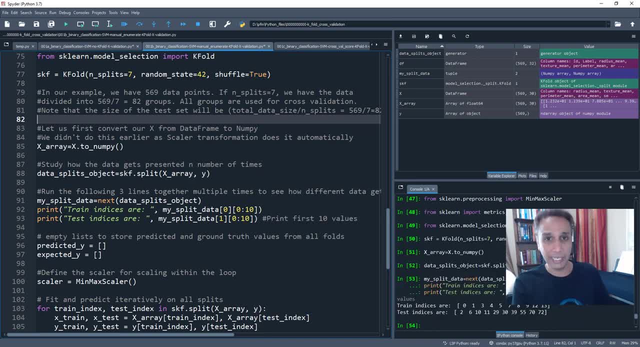 i'm just uh of the first split. i'm just looking at the first 10 data points and you can see the train indices are zero, one, three, four, five, six, seven, eight, nine. so two is missing there, six is missing, ten is missing because they are available as part of test. yeah, so, uh, that's uh the indices right there, and why is it not continuous? 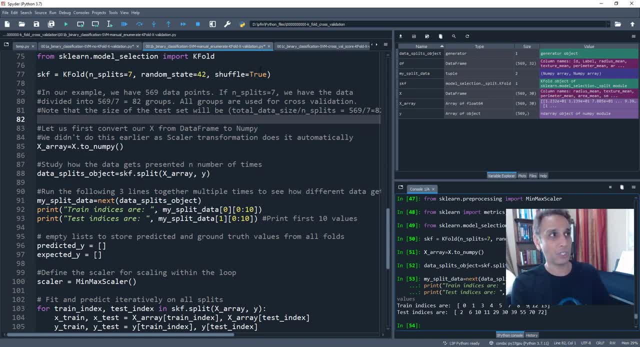 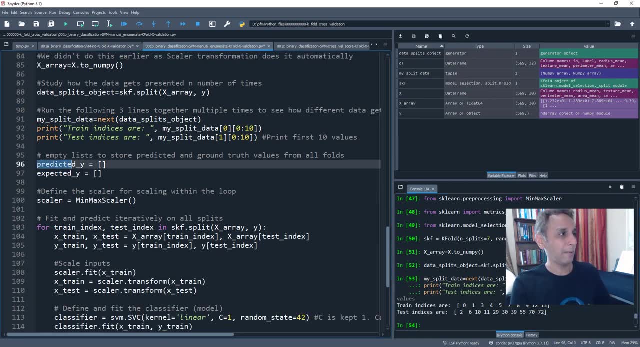 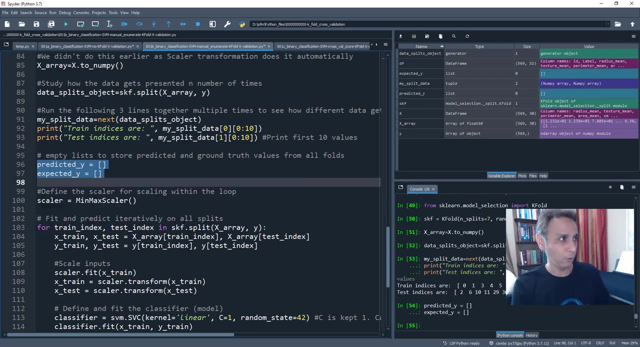 zero to fifty and then so on. that's because we uh put shuffle equals to true. i hope that makes sense, okay. so now let's uh create a couple of empty lists because we want to capture the predicted and expected yeah, so we can do the accuracy for each fold. so i created an empty list right there. we also define our scalar as min max scalar. 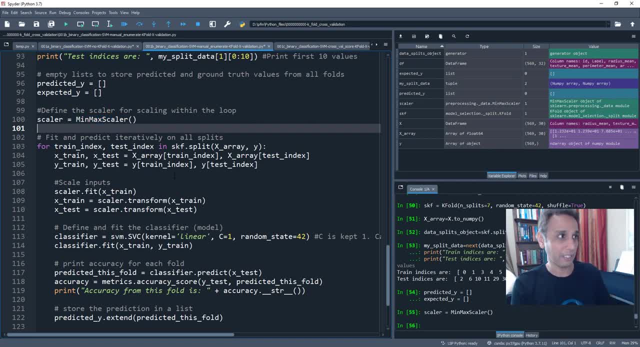 and we'll be scaling inside the loop once the split happens. and how does the split happen? so, for train index and test index, remember, the split is going to give us the indices. the split is giving us the indices right there: zeroth, first, second, third, right. so so, 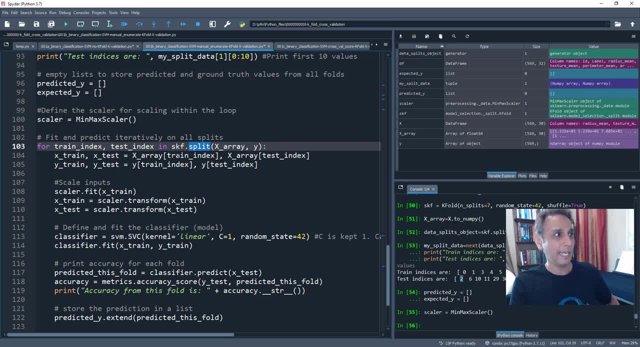 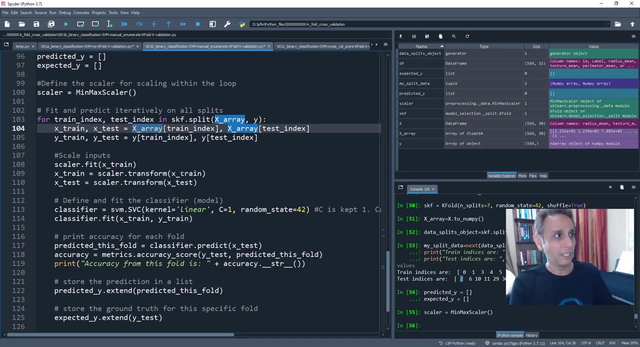 we go through each of those indices and then we get our x array and we get our uh for our train and test, and we also get exactly the same for our uh, y values, the pred uh, you know, and then we are going to do our fit right here for train and test. we are going to transform them, we are 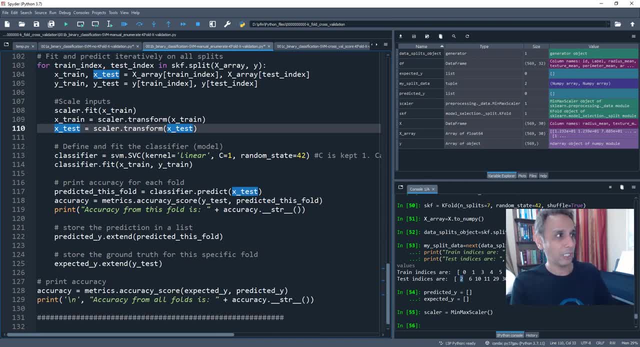 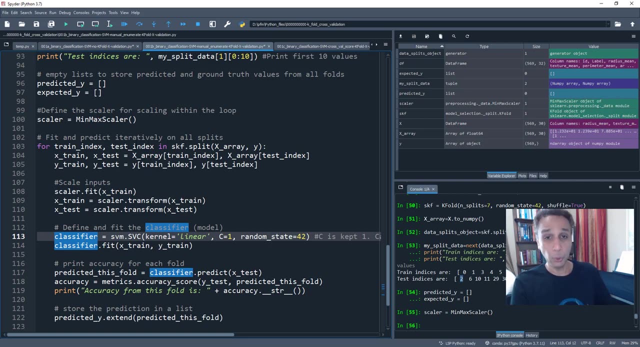 going to apply the min max scalar and then we are going to do a uh training on on this data. first we find a classifier and then we fit right on our x train and y train and this x-ray and y-train it changes for each loop right here, so it's manually enumerating through each group of these 83 groups. 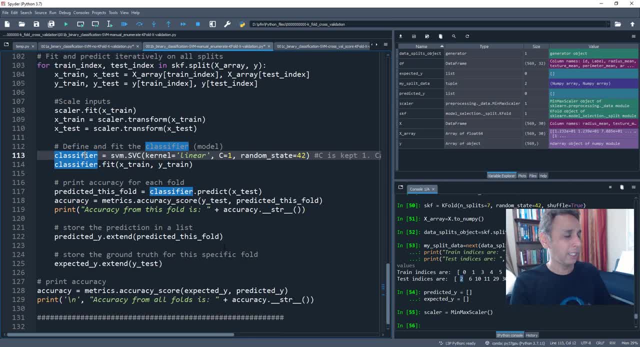 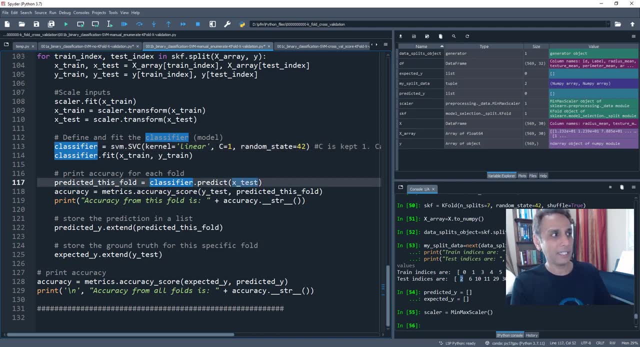 that we just uh, create, uh, by doing this split, okay, and of course, uh, once the model is trained, then we need to predict. and how do you do classifier dot predict on your test data set? so that's the predicted for this fold, for this fold, that's the predicted, and i want to 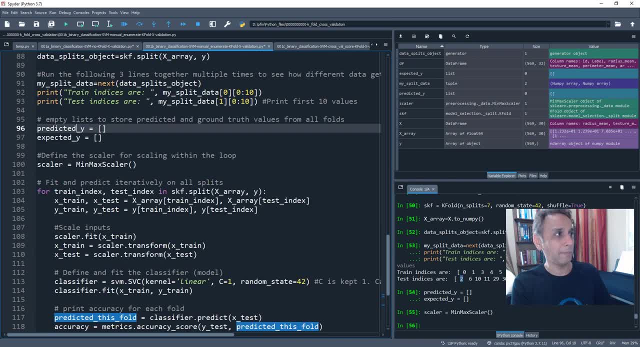 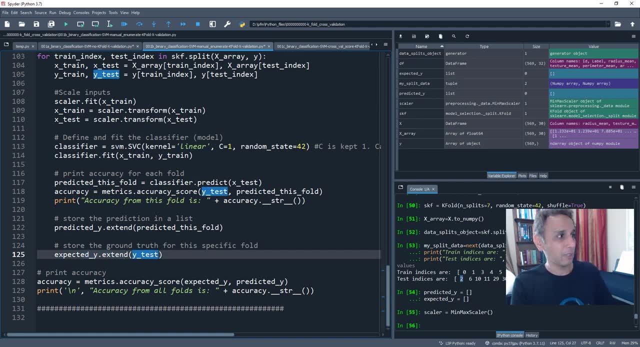 capture that as part of uh, as part of our empty list right there, and i would also capture the expected value, which is nothing but our y test values, and of course i'm also calculating the accuracy, which is matrix dot accuracy score, between your test and the prediction, and i'm 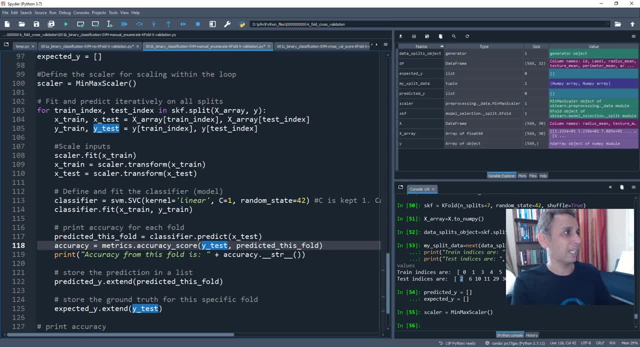 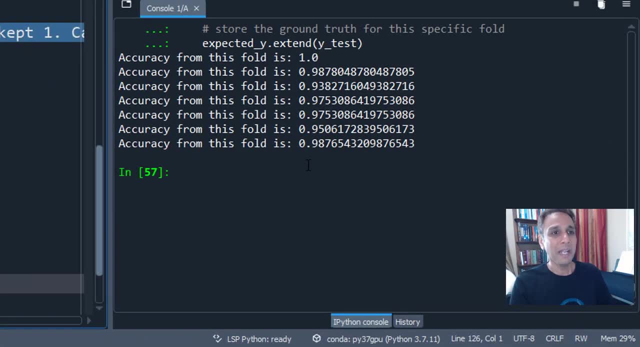 going to print that out, okay. so let's do all of that. it should be pretty fast, it shouldn't take that long. let's go ahead and run it. so there you go. so apparently my first fold. the accuracy is one. the second 100, second fold: 98.8 94, 93, 97, 97, 95 98. there you go, and if you want, you can actually. 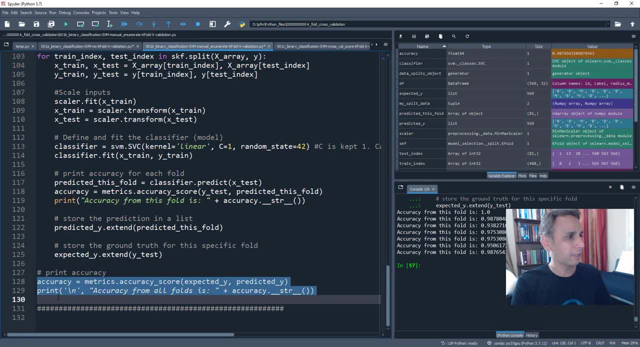 average, all of those uh, uh, let's see what am i doing here. oh, i'm just printing the accuracy right there. sorry, not average, but uh, accuracy score expected, predicted right there. and when you do that it's giving me ninety seven point. uh, three, six, three, uh, what am i? uh, i. 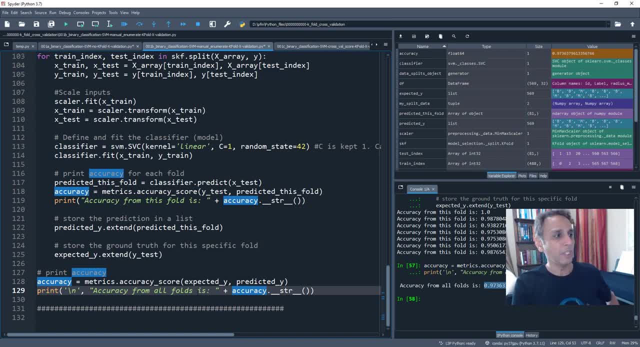 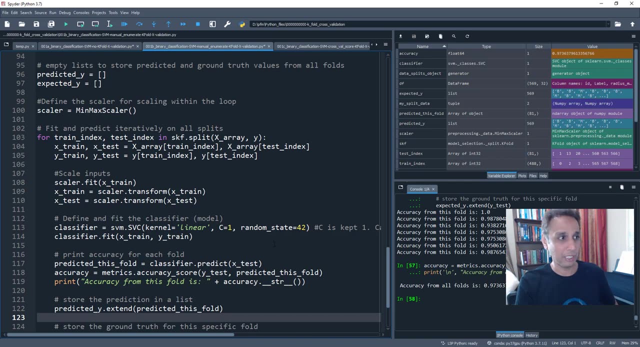 sorry, i should have uh been prepared. oh, from all folds. yeah, so this is the accuracy from all folds. uh, there you go. we are getting uh 97, point. uh, whatever that value is. so this tells me how well my support vector machines is working. with a c value equals to one and random state equals to 42. 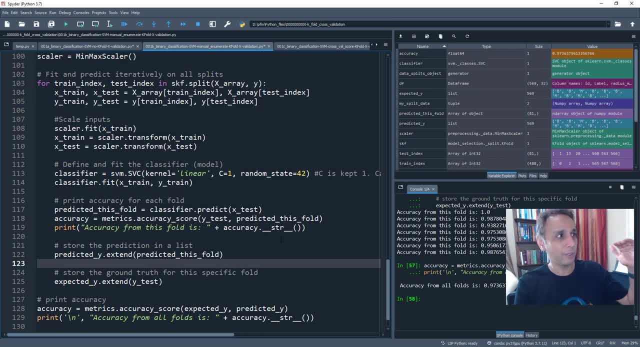 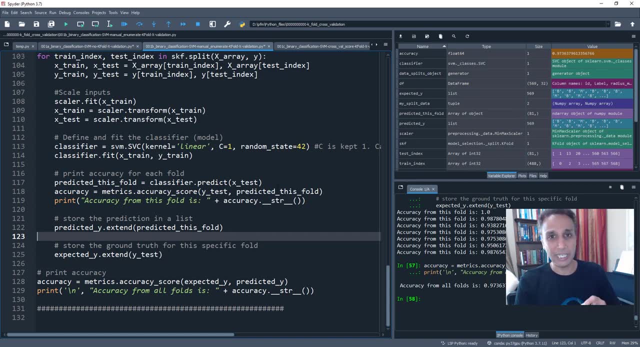 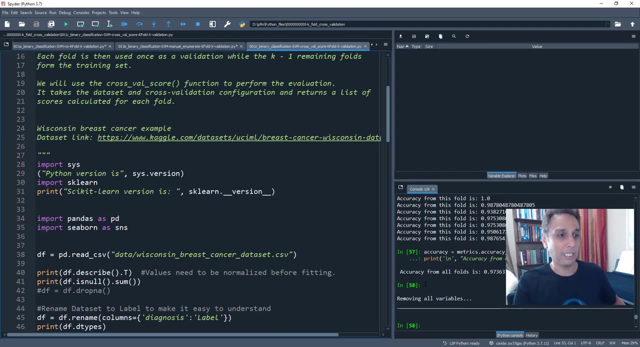 but random state. you can change it, but this tells me how the the model is working on this data set. now we enumerated all of this, but it's very easy again. let me end the video by showing you how easy it is to just use a built-in uh method. 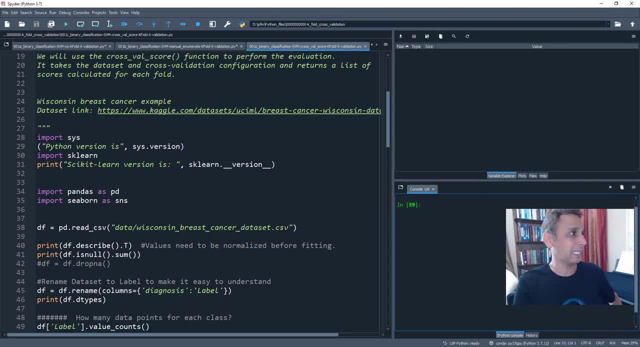 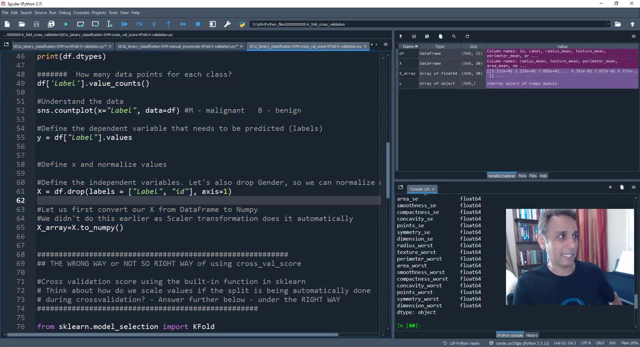 so let's clear everything here and again. i'll do exactly the same i've done before. run these lines all the way to right here. yeah, remember, we converted our x to our array numpy array. now what? so how do we do this right away? so the trick lies: 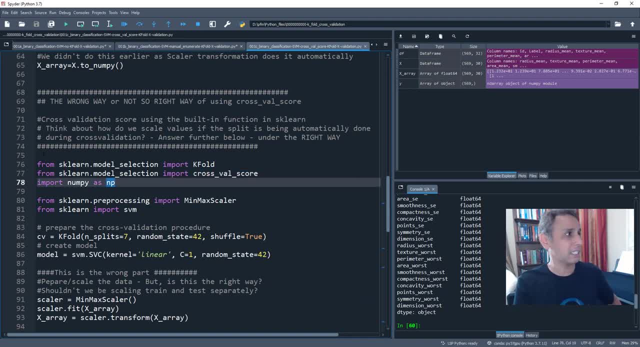 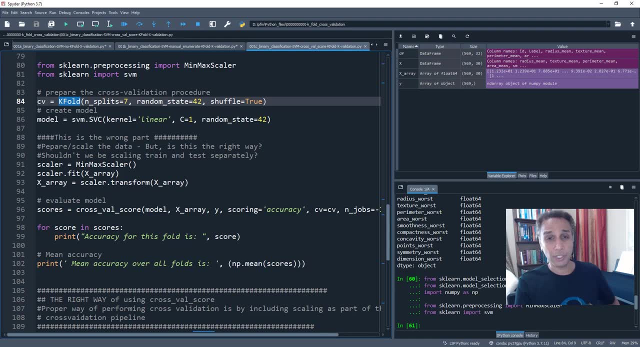 a here cross val score as part of scikit-learn model selection. so let's go ahead and run all of these and now prepare the cross validation procedure. so how do you prepare the cross validation? again, exactly same as before. number of split: seven random state shuffle equals to true. 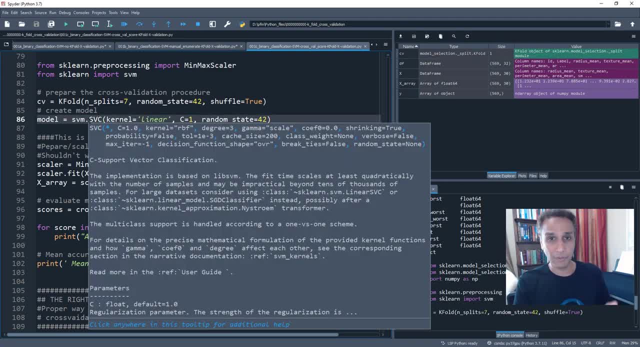 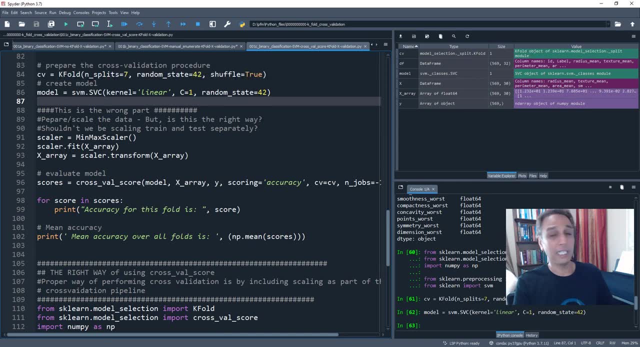 let's go ahead and do that. and what is our model? our model is support vector machine with these parameters. go ahead and do that. and now i am uh defining my, uh, you know my, my uh- scalar and then scale the values. but this is the wrong way. you know that i already. 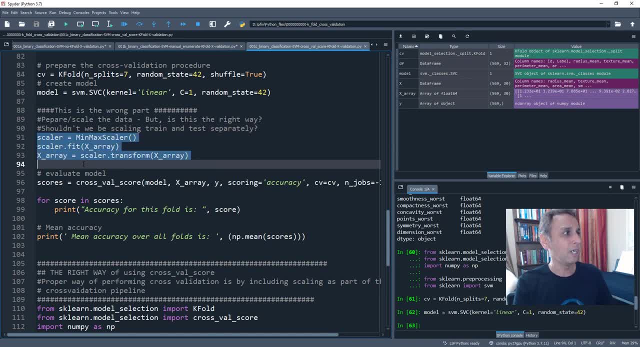 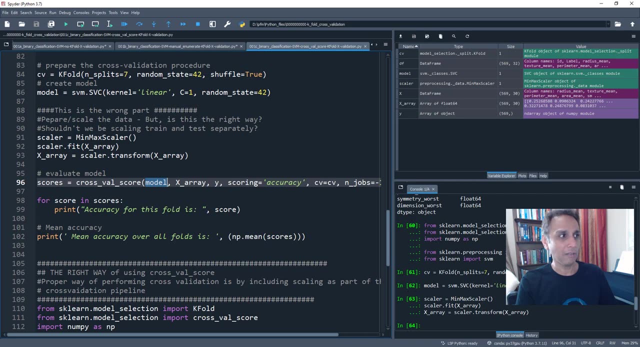 mentioned about it. you do not want to scale the values before uh and then uh print it out. but if you do that, again we cannot tell that it's wrong just by looking at this. if you do that, the way you do apply your cross validation score is you provide a model. which model do you want to use? 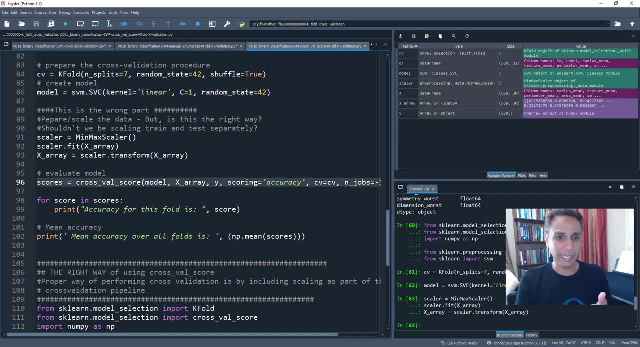 we want to use this one, and you provide your x values and you provide your y, and what is your metric that you want to report score in? in my case, i want that to be accuracy, and what cross validation process do you want to use as part of your cross validation score? we already defined this up here. we want to use this, and 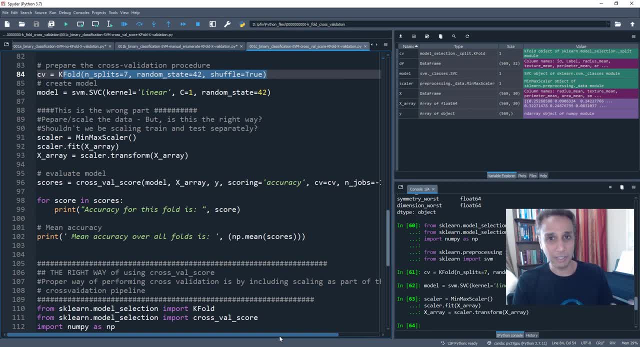 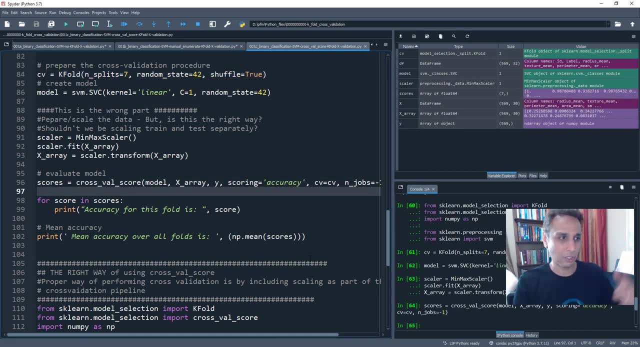 number of jobs equals to minus one. it parallelizes the, the calculation right there. so that is it. this is how you use it and scores. it takes a while, it needs to go through all of that, and now let's go ahead and print the accuracy, uh for each fold and the other one, and then we're going to go ahead and 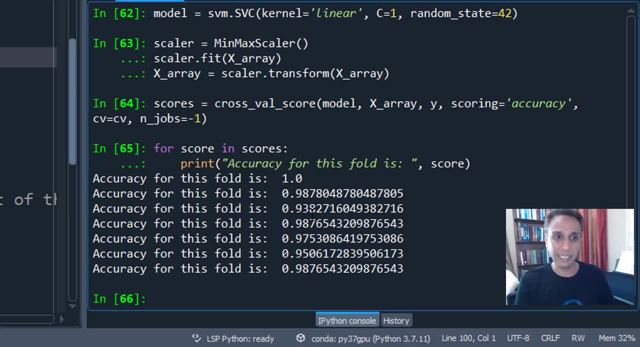 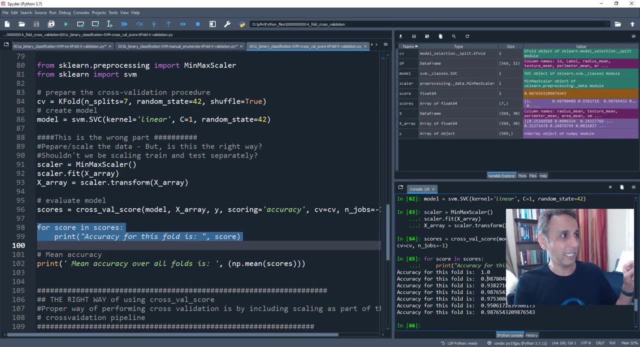 print the accuracy, uh, for each fold and the other one, and then we're going to go ahead and print the accuracy and it's very similar to what we got before, right, 100, 98, 93 and so on. but again, like i said, this is not the right way to do it. the right way to do it is by actually scaling it. 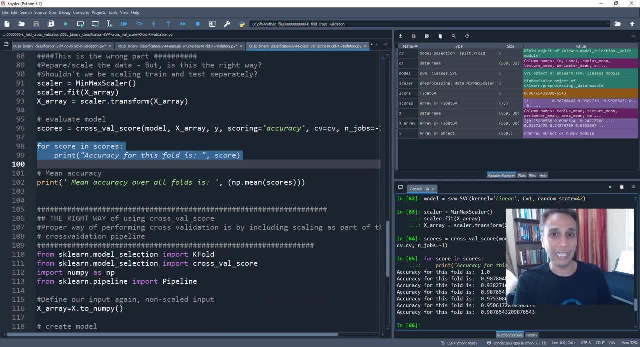 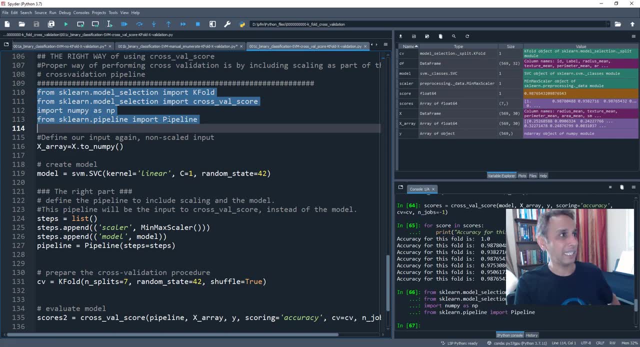 inside, here, inside your cross validation, and how do you do that? and let me end the video by showing you the right way to doing it. so let's import all of these libraries again, and the key one here is the pipeline scikit-learnpipeline import pipeline. yeah, and 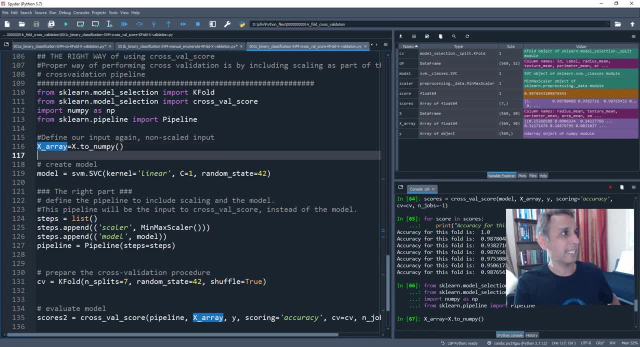 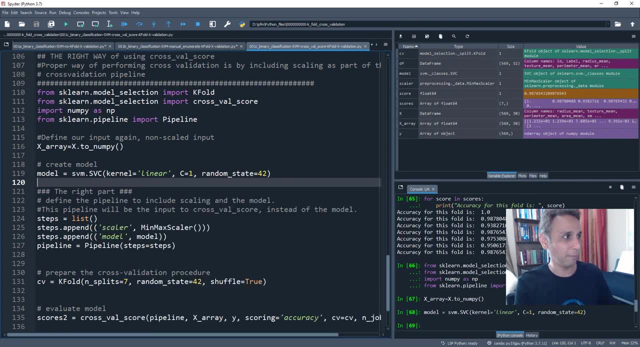 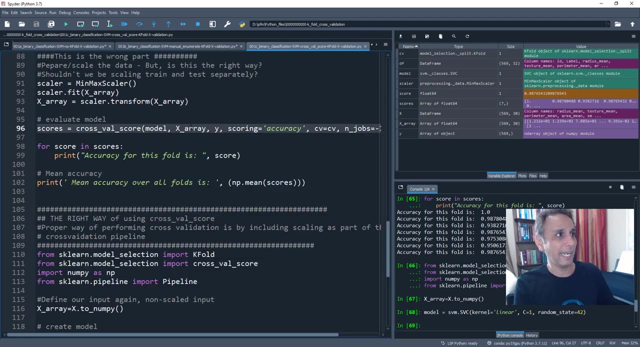 uh again. let's convert our x. uh. let's get our x array again and let's define our model: equals to support vector machines. we know this is exactly what we did before. the key difference now, what we are trying to do here is: instead of just providing, instead of just providing my model. 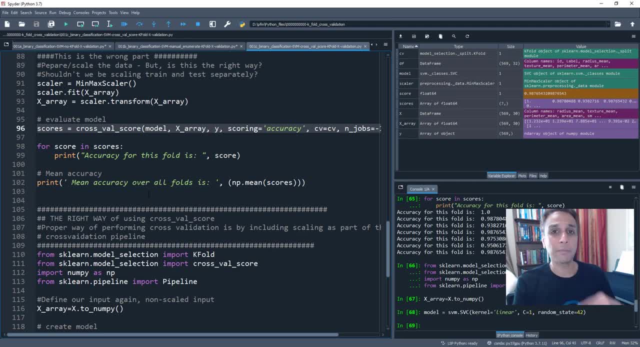 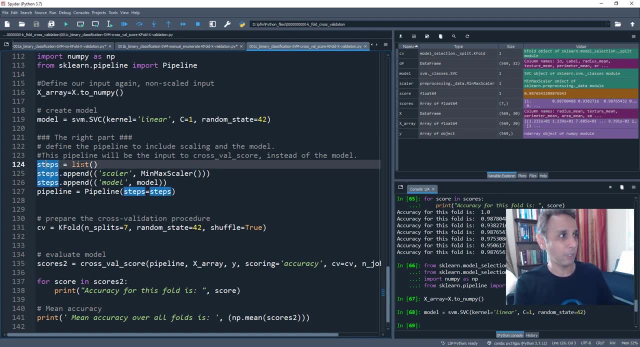 and x and y and all of these. i'm going to create something called a pipeline, and the pipeline is created first. let's give a- you know, variable steps equal to a list. i'm just creating a list, yeah, a list of what, a list of my scalar, what scalar to use and what model to use, and then i create a. 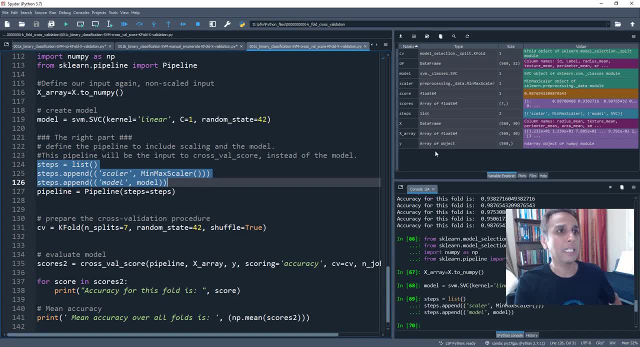 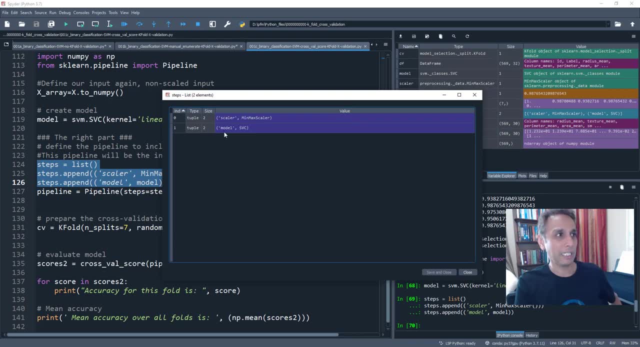 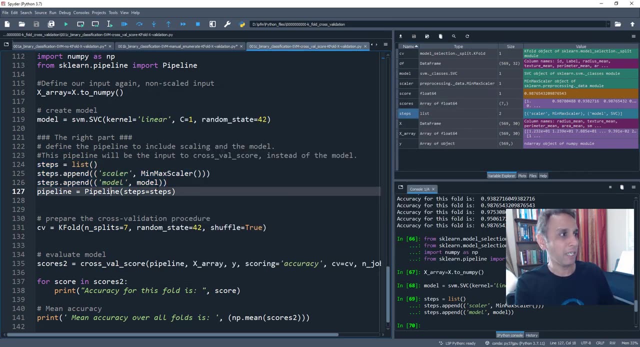 pipeline. so if i run these the steps is nothing but a list right there showing us. this is a tuple of size two scalar min, max, scalar model support vector machine and if you want more, you can go ahead and add more and i'm going to create my pipeline with these steps. okay, i created a. 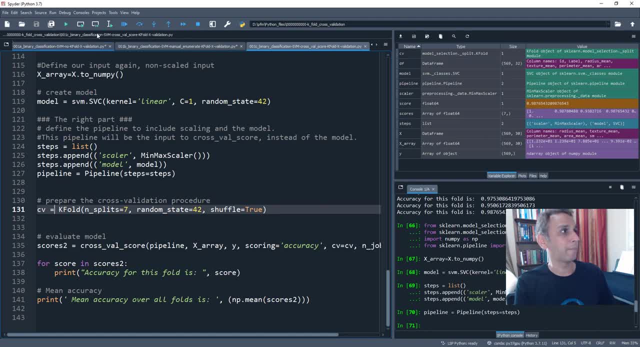 pipeline. rest of the story is the same. so i'm going to create my pipeline with these steps same. i create my setting for cross validation and let's go ahead and do the scores again. i gave it new value so we can compare with the other one, but here, instead of the model, i gave it a pipeline and 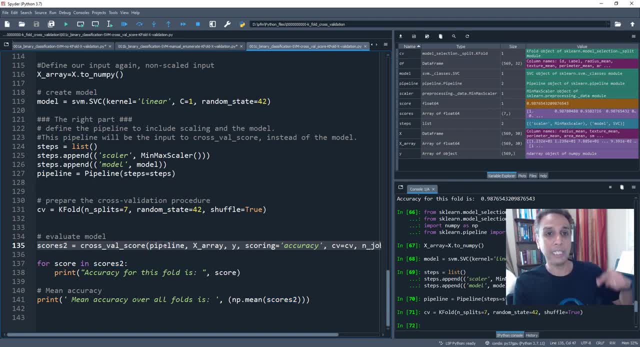 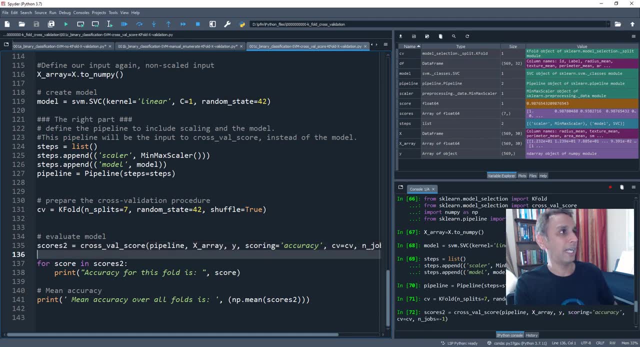 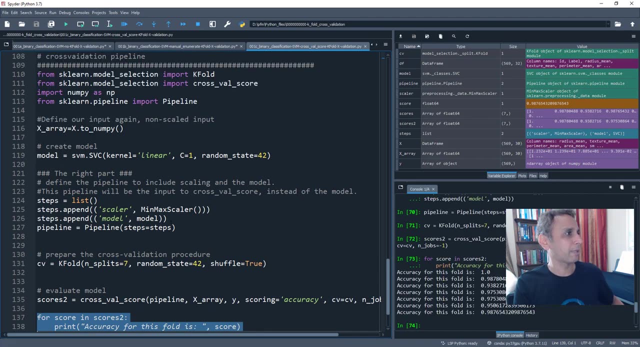 then this is the input x, this is the input y and, as part of the pipeline, it takes care of this. uh, this part of the min max scalar part. so let's run this and print out the scores right here and also print out the scores from before. yeah, just so we can compare them. 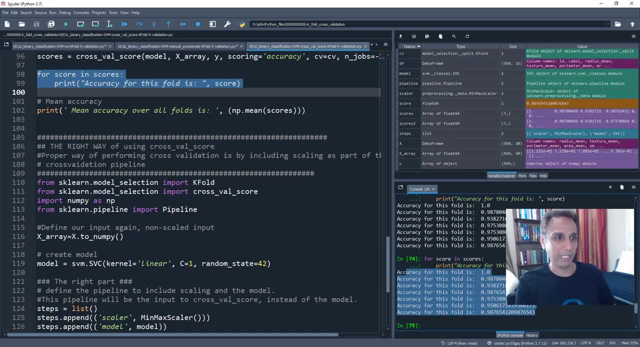 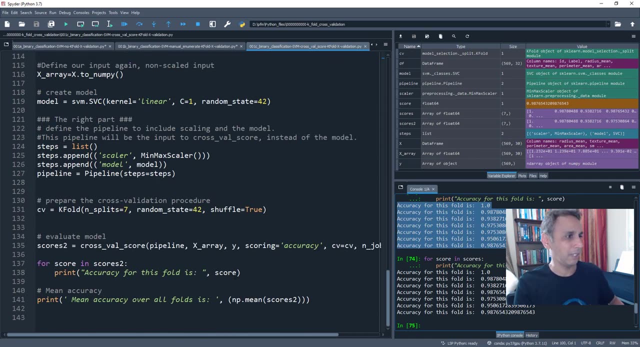 there. so this is the wrong way of doing it. this is the right way of doing it. i mean, in this specific example, they look almost identical, but uh, but, uh, it it's again, it it may be different, uh, you know, for for different types of data, in fact, am i doing the same? oh sorry.